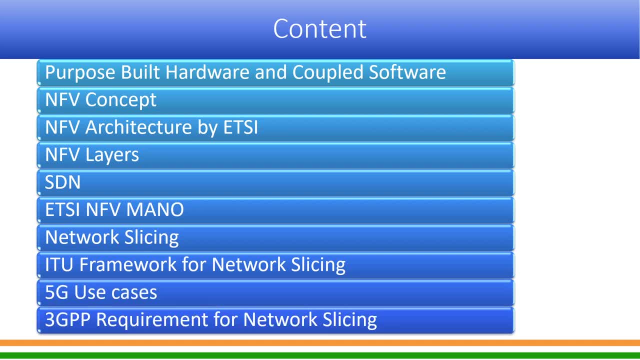 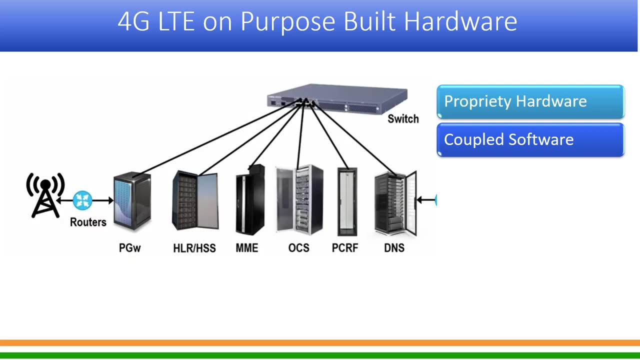 at that, and then what are different use cases? and then 3GPP requirements are also there for slicing. So this is the content. we will try to cover it today. So let us look at 4G networks. In a 4G network, if you look. 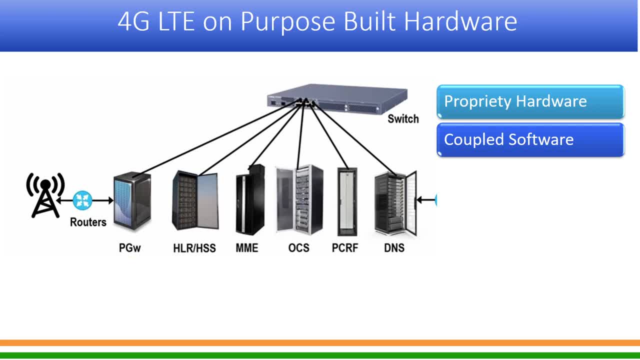 at the actual network element. they look something like this, although they will be located in some server location and all, but it will look like this. So you have boxes for, say, PDN gateway. you have boxes boxes for MME- mobility management entity. 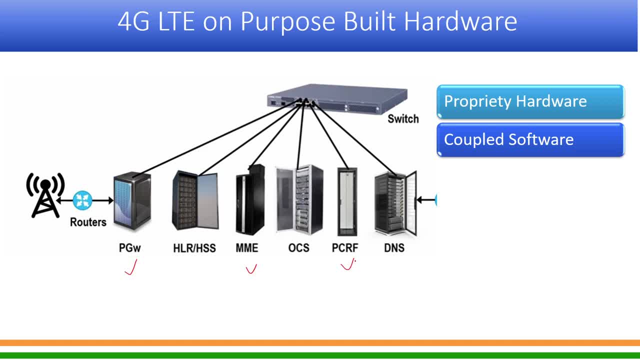 you have a certain box and policy control function, etcetera. So for every functionality you have a different box, which is kind of a purpose built hardware, and it is a coupled with a software. So what is the problem in this particular kind of purpose built hardware and software? The problem is that you are kind of 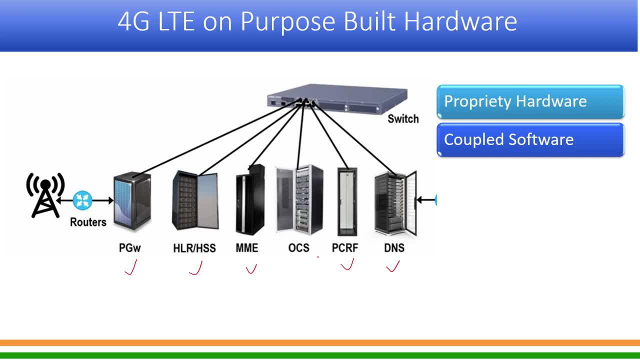 if you have bought a, say, 4G equipment from, say, one vendor X vendor, say Nokia or Ericsson. So whenever you want to expand either a single element, the same element or overall, you have to go back to the same vendor, Even the expansion in the same. 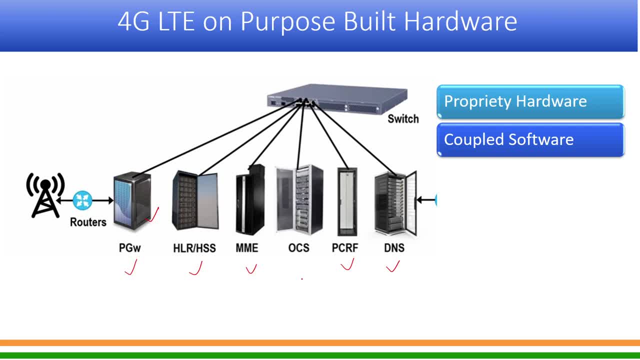 box. you cannot buy it from other vendors. You are locked to a particular OEM or otherwise. if you want to change the OEM then you have to do almost replace everything. For example, so the BSNL, when they procure some time to open tender, L1 becomes some other vendor, like if earlier they. 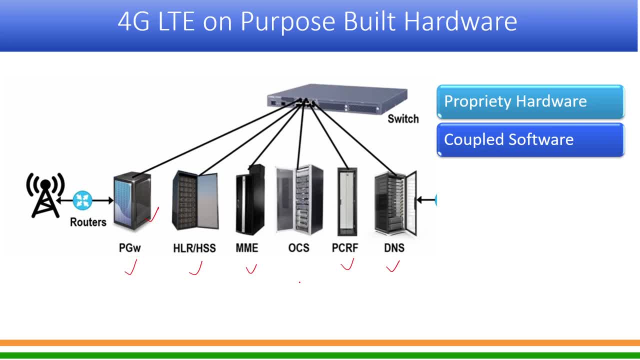 have a network of Nokia. this time they will. they may have network from Ericsson. So they have to plan. in one zone they shift one type of equipment, in other zone they bring in the new equipment. So a lot of re-engineering is required. So that is an issue that you are kind of tied up with. 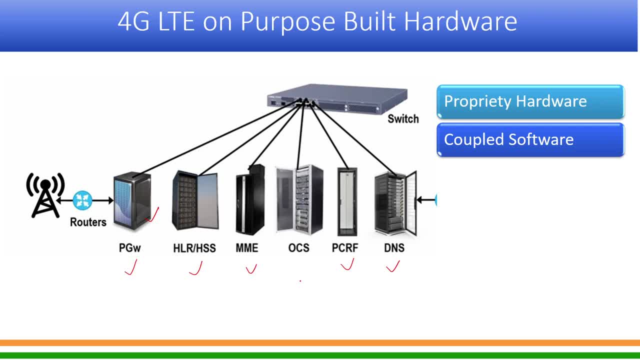 one vendor and then for a small expansion, that vendor may charge you very, very high cost. That is a practical problem with a purpose built hardware which is till 4G. it is the situation but in 5G, as we have discussed, based on service based architecture and hardware software. 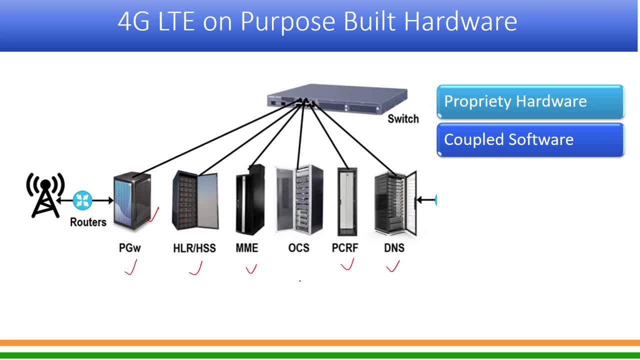 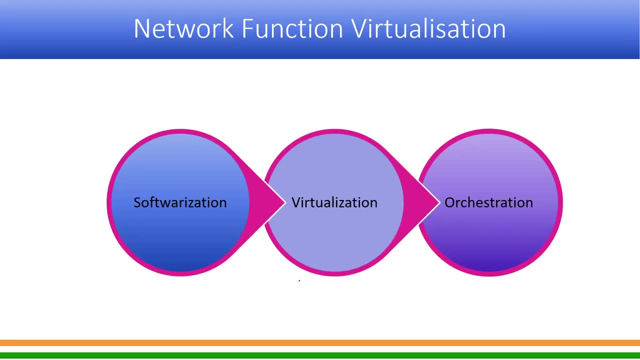 desegregation and the network becoming a software function. There is a possibility of a request to mute your mic. I think there is some background noise. Thank you. So what is network function? virtualization, broadly. So it has got three components. when we virtualize your 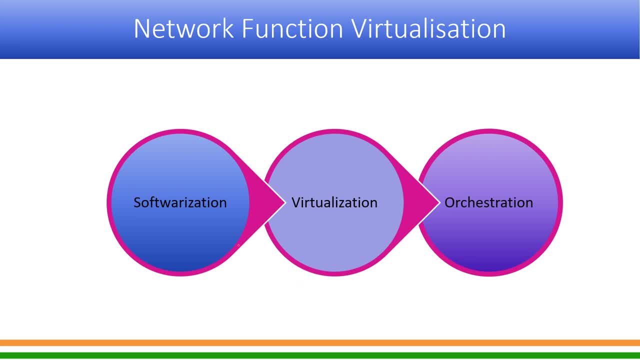 network functions. So you have to do three things. The first is the softwareization. that means those network functions. for example, in case of 5G, be it AMF or be it SMF or be it PCF, we have to softwareize those network function from a purpose built hardware and coupled software. 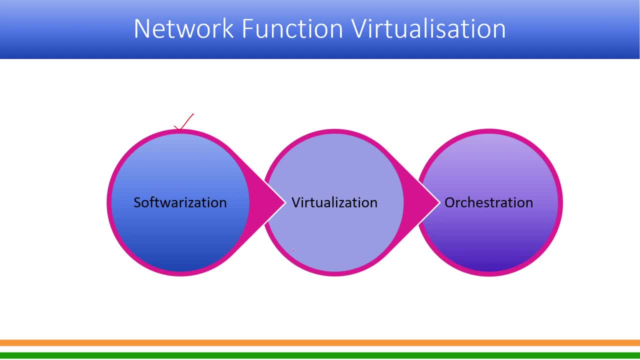 you to make a network function a virtual network function, and then you have to virtualize. that means virtualized environment. now you don't need a kind of a purpose-built hardware or a specific hardware. you can deploy that on a virtualized environment, on a COTS environment. COTS is commercially of the 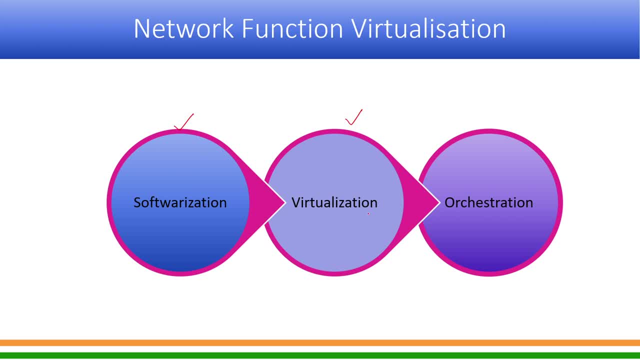 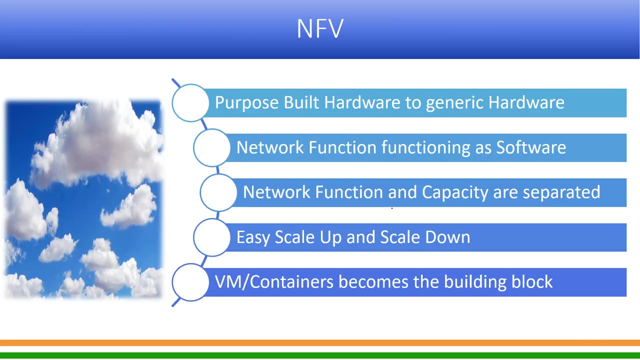 self servers. and then, once you have deployed your software network function on a virtualized environment, you have to manage that, orchestrate that. so you require a manual management and orchestration environment which will manage all these virtualized network functions. there are broadly three components which has to be managed. so what we understood that, what is NFV? 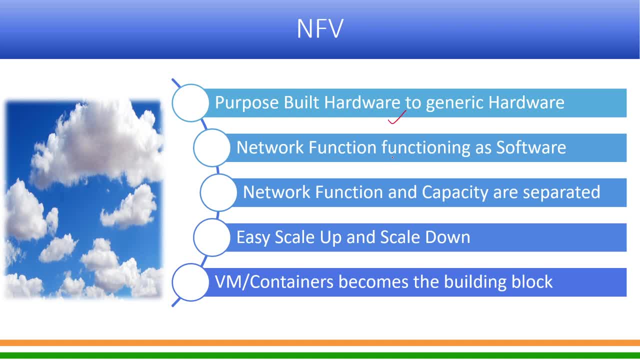 NFV is nothing but from moving from a purpose-built hardware to a generic hardware. now you can use any company's server, be it Dell, be it HP, or you can buy from any company of the self company of the self hardware, and then your network functions once. 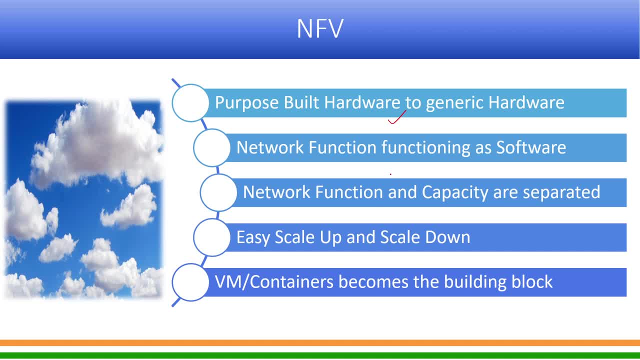 you are able to deploy a network function on a generic hardware, your network function has to become a software right, a piece of software, a virtual network function. so that means your network function and the capacity are separated. what does this mean? is that earlier, when you had or when you have to expand your HLR, you have to completely expand. now your network function is 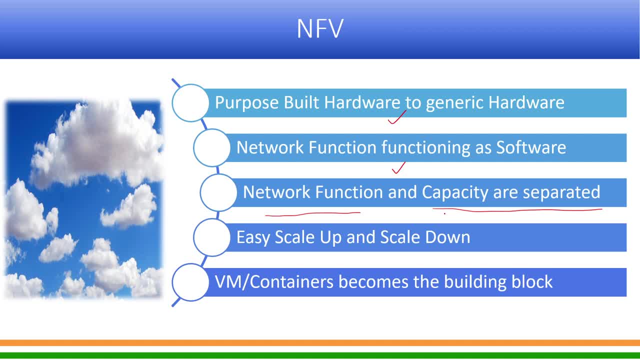 a different part, and capacity is just: you have to increase your compute, increase your memory, increase your networking elements right, so that way you can separately increase the capacity. so network function and capacity become separated. you can easily scale up or scale down. what I mean here is that, suppose. 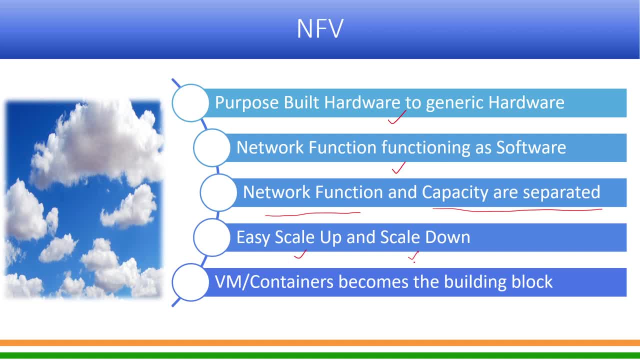 you have a less traffic. so suppose you have multiple instances of AMF running onto your hardware but you feel that number of customers have gone down in a particular area or you have a less load. so you can- I mean, scale down easily. you have to just go: software function, you have to. 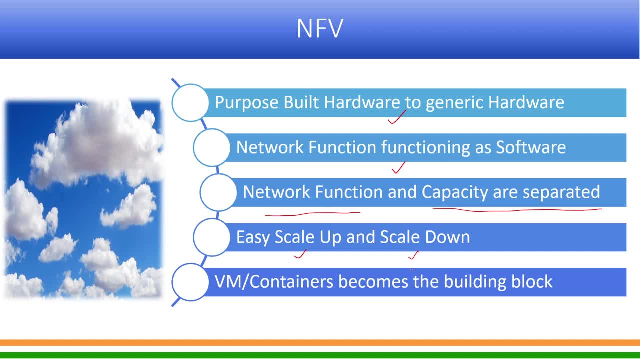 remove or modify and scale down. you can save on power, you can save on other resources. similarly, scaling up would also be easier that you have to, you can. you can create a new instance of a particular network element. if traffic is growing in any area, and then so in in all these scenario. so what becomes a building block for? 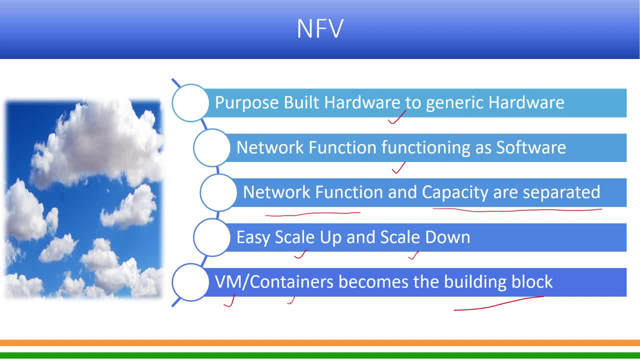 us is the virtual machine, or containers so on, a virtualized environment. when your physical resources like servers, compute or memory or network becomes a virtualized environment, on top of that you can deploy your virtual machines you be aware of, or there is a concept of container within the container, you can deploy any network. 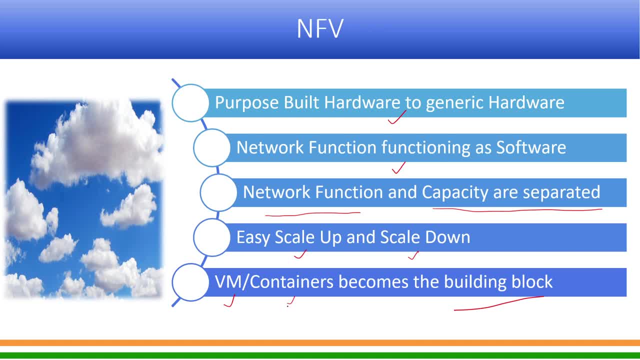 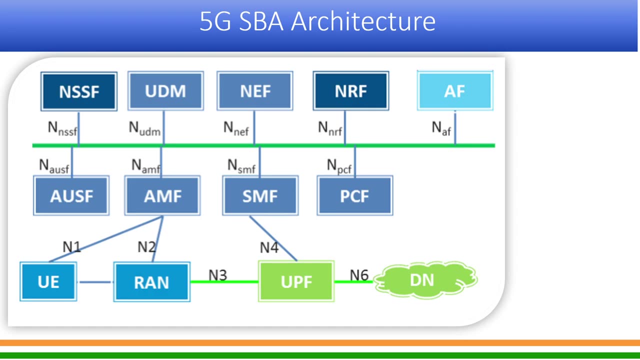 function or any application, So that becomes our building block for NFV. So in Nutshell, these are the changes when you bring in the network function virtualization into your network. So when the 5G network architecture was being created by 3GPP, they kept in their mind that. 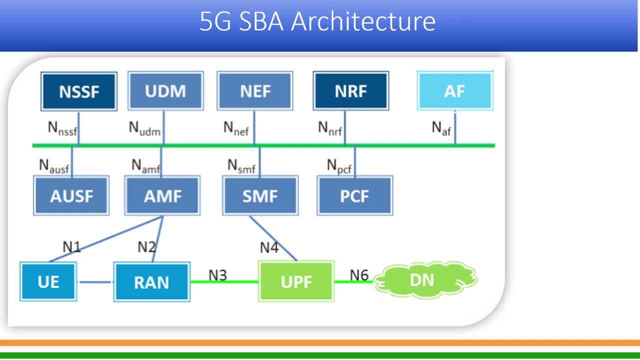 the network function which they are specification, for, which they are creating, will be deployed on a NFV infrastructure. So, accordingly, from earlier a reference point architecture- reference point architecture they I mean change to a service based architecture where all those aspects are taken care. So there is one question which 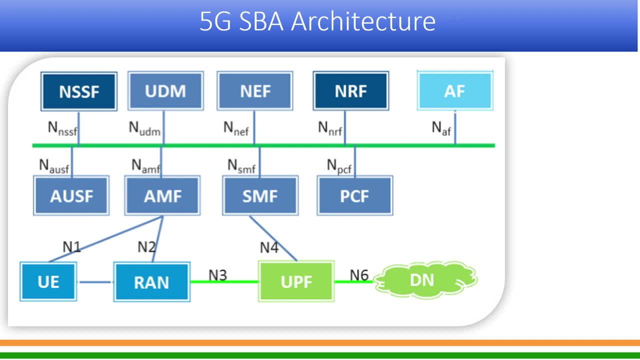 has come on to the chat box, that is, a scaling up or down, or which module controls it? That is a very, very good question, Kiran. So answer as of now here is yes, The scaling up or scaling down of a network can be made automatic if 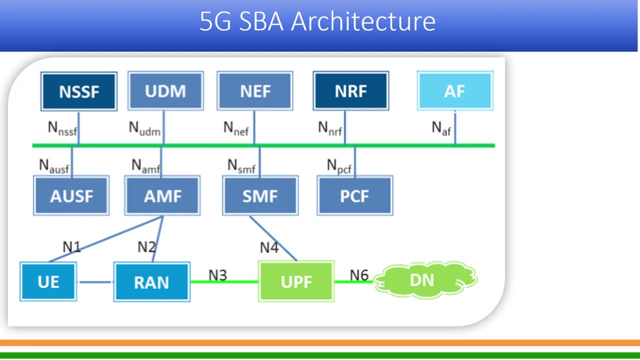 we deploy the network function on a container and we have a MANO Management and Orchestration and we have already defined the configuration that suppose, if a traffic increases from this threshold value to this threshold value, please create one more instance of, say, MF or SMF. 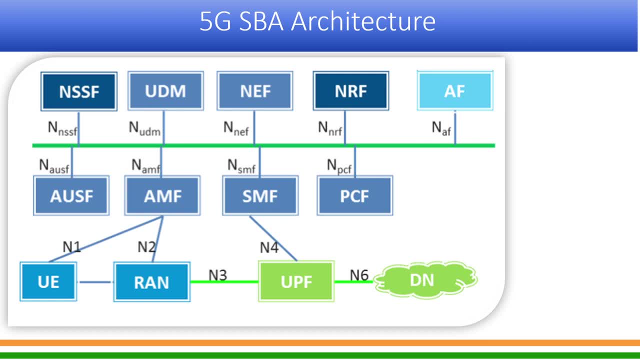 and vice versa. or even if a particular network function is giving trouble, then that can be set down and new instance can be created, So that becomes automatic based on the configuration, which you have done while, basically, while rolling out your network. So I think you 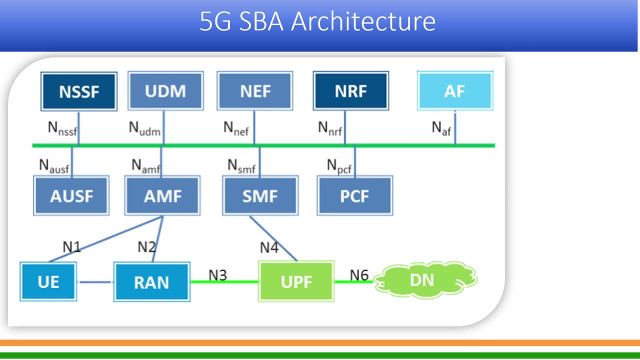 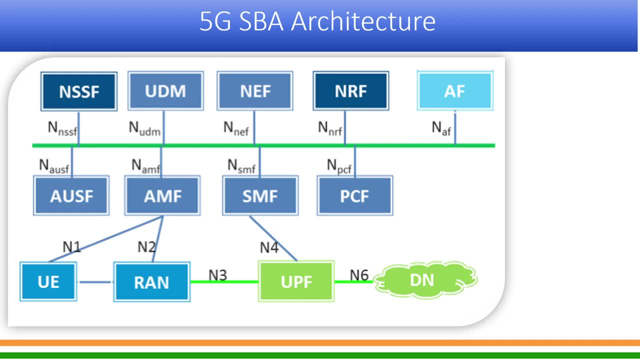 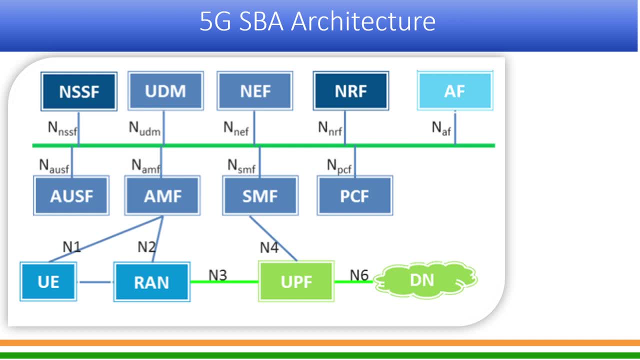 software you do a MANO Management and Orchestration. So there you can configure all these aspects and accordingly those automatic creation and modification or deletion can take place. So what we are looking at, that these network function, has become a virtualized network. 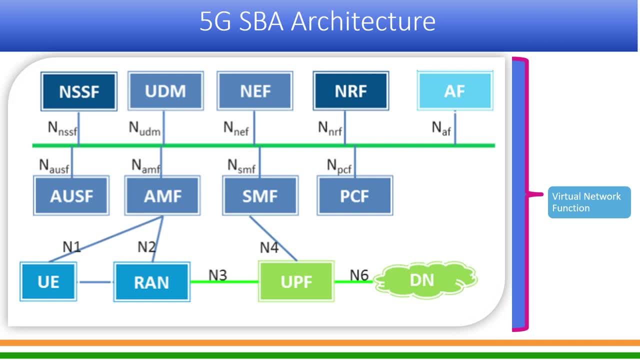 function. So in 5G SBA architecture all these network function or most of it. So there is a possibility that even you can have a mix some of the network function as a virtualized network function. some of the network function can still be working on a bare metal or a purpose built. 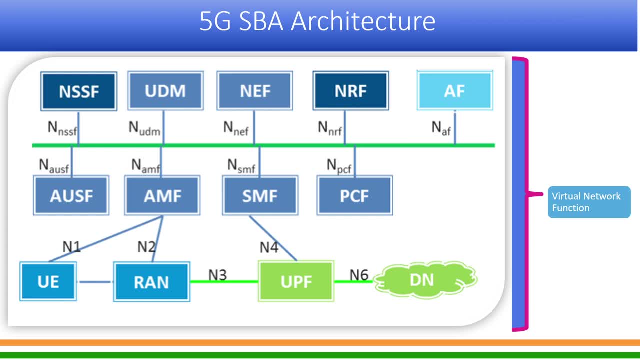 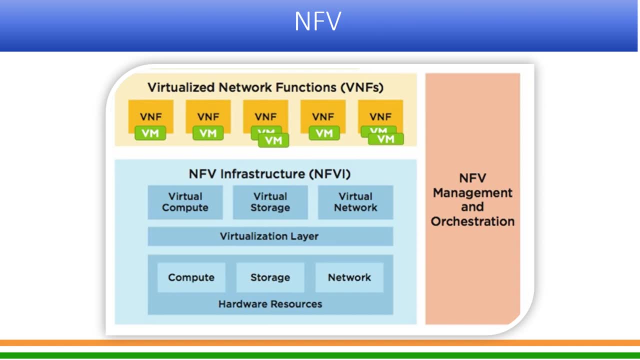 hardware and software Mix and match would be possible because interfaces are open. So, as I said that our presentation is based on itsy-itsy, So let us take a look at the architecture of NFB. So I had shown you the initial URL. 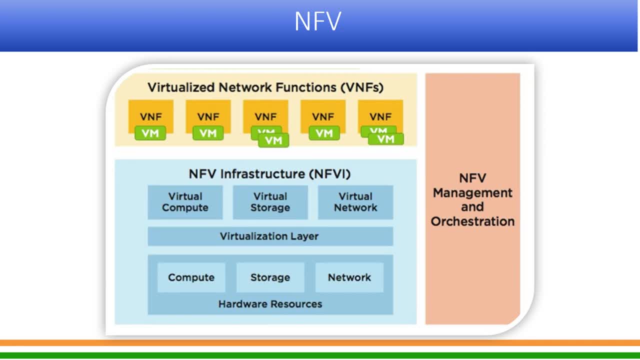 from where you can get the document. rather, I shared 3 documents on to the WhatsApp. one is the architecture, other is some use cases of NFB that was worked out by the itsy itself, so you can go through that in your leisure time. So how it works, I will just explain. 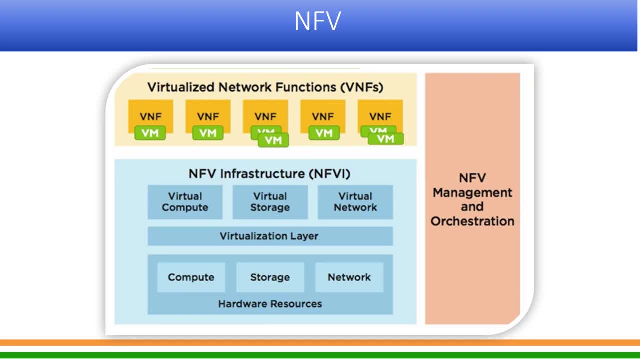 broadly that when we say and then be what we mean. So all those hardware resources. I said that software becomes disaggregated, so your hardware resources, see, see here, your hardware resources. so what are those hardware resources that can be your servers, memory network, so basically compute. 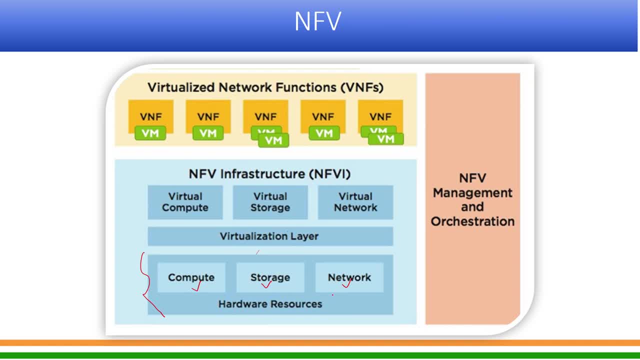 storage and the network. so using some virtualization software like vmware or any kind of other hypervisor that is, you can virtualize these compute, storage and network. so when you virtualize, that means dynamically- you can allocate these resources, some compute to some compute, some storage and network elements to one virtual machine, other virtual machine or 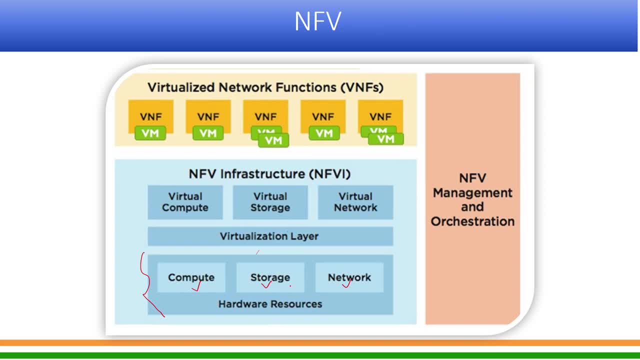 fourth, virtual machine. so basically you are creating virtual compute, virtual storage and virtual network. so this portion is called nfbi, this network, this is called nfbi, nfv infrastructure. on top of this, on top of nfv infrastructure, now there is a possibility that i can deploy virtual machines, vms. so those who are from 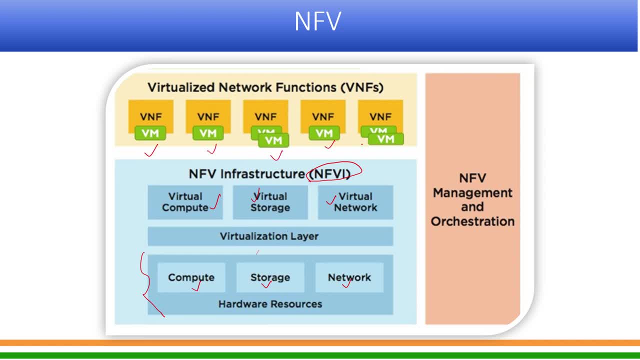 it background will understand better that you can create virtual machines or you can create even container. so here in this example it is virtual machine which has been shown and on top of virtual machines you can either deploy one virtual network function, your network function, virtualized, or even more than one you can deploy, or in more than one bms one bnf can be deployed. so it's a very 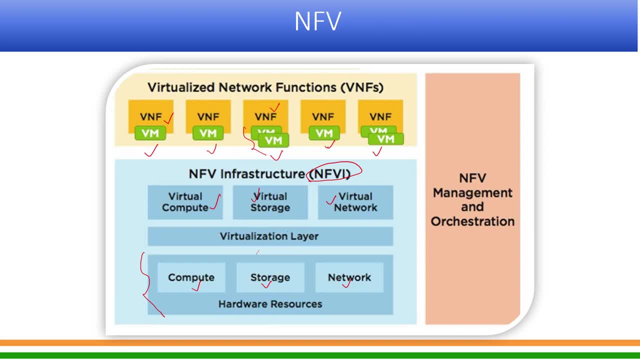 very dynamic configuration which you can do, that one or more than one virtual machines, you deploy virtual network functions. so this is how your nfb looks like. on to the right side, what you see is the mano part. how will you manage this nfb infrastructure or or those virtual machines or 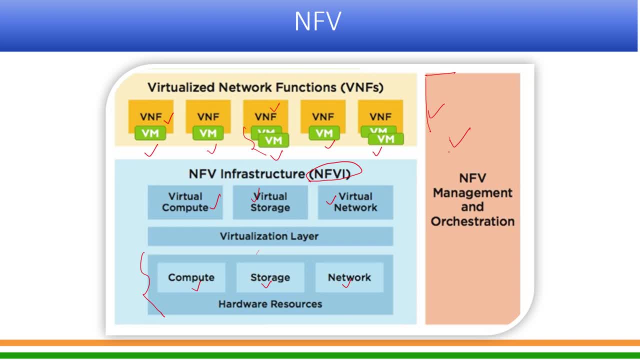 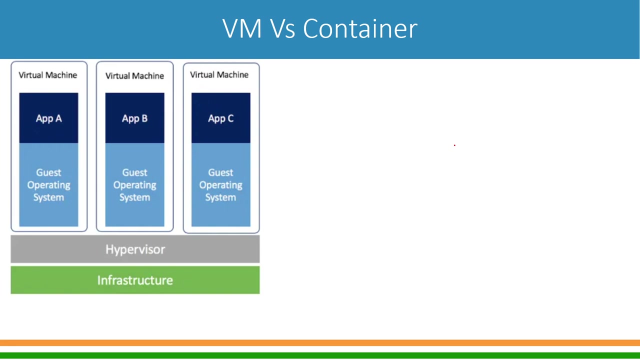 virtual network functions is a function of nfb. this is also a kind of software which will manage all these aspects which we will talk about in upcoming slides. so this is called nfb management and orchestration, mano, in short form, mano. so let us just discuss about what is virtual machine and what is container. for those who are, 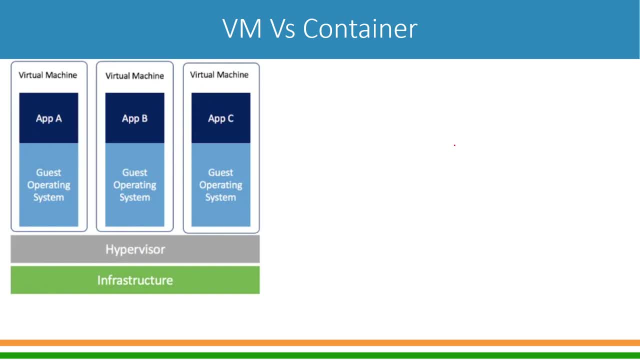 not from the it world and have some idea about computers working. those in it world would already be knowing it. so, basically, the when we say virtual machine, what happens is that once you have your infrastructure- infrastructure where i mean your servers, your compute, your storage, your networking- you can create multiple virtual machines using any hypervisor. that is a kind of a software, vmware or 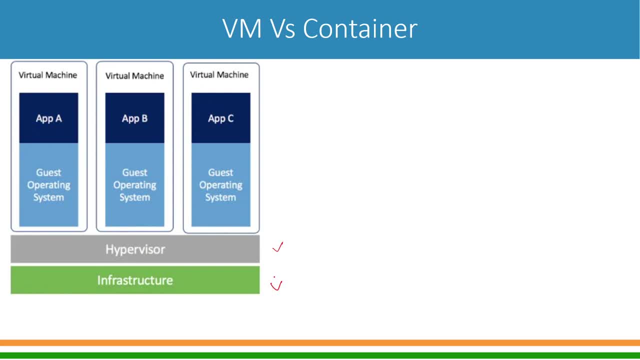 there are many such software. you can create multiple virtual machines. for example, if i take example of your laptop, if i deploy a hypervisor on top of your laptop, i can create two, three virtual machines. so small vm can be created. similarly for servers. on servers, you can create multiple virtual. 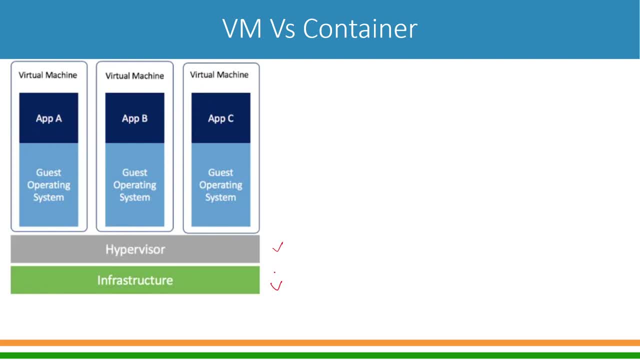 machines. so when you a virtual machine basically, then you again load a operating system onto the virtual machine. so those are kind of a guest operating system. so every virtual machine can have different operating system and top of that operating system you can deploy those applications. this could be. 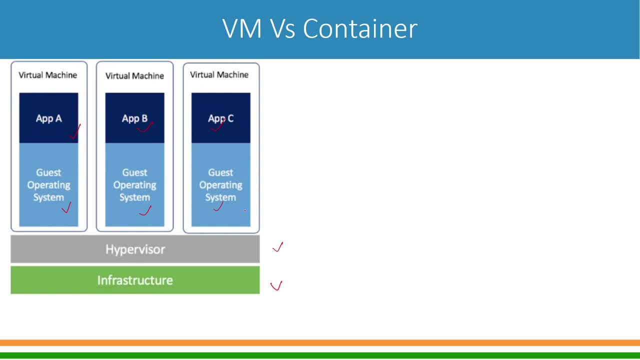 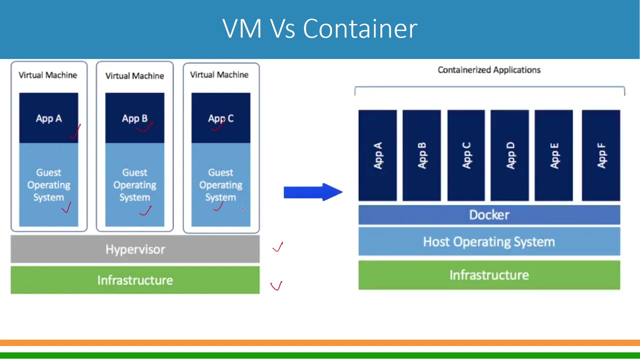 your virtual network function or any, any application. this is a way i mean virtual machines. even today, a lot of such environments are existing across the it world. but nowadays, instead of virtual months machines, we- i mean industry- has gone for containers. for its i mean better efficiency and better management. so what is? what is those container? so if you move from a vm 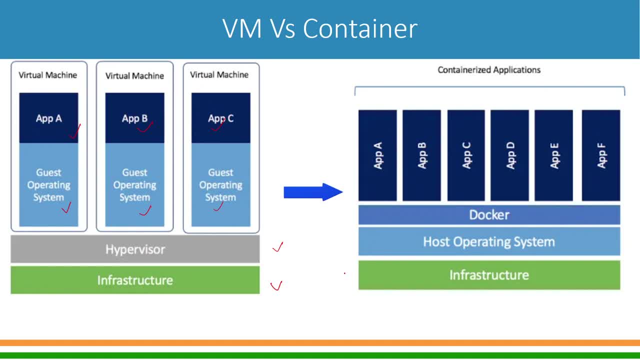 to container. you can just see this picture and again you have a infrastructure that is, your servers, your memories etc. onto that you have a host operating system, so basic kernel would be running here, and on top of that you deploy a software like docker. there can be some other software also which containerize. i mean using 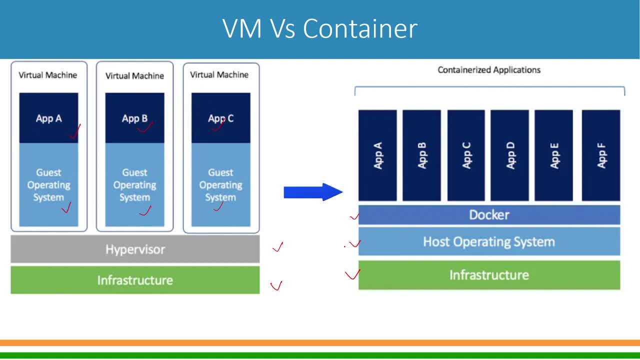 which you can create a container, uh, environment, right. so when we say so, these are containers, so one container having one app, second container, third container, fourth container, and so on. so multiple number of containers can be deployed. so it becomes more flexible, uh, and you can, you can. 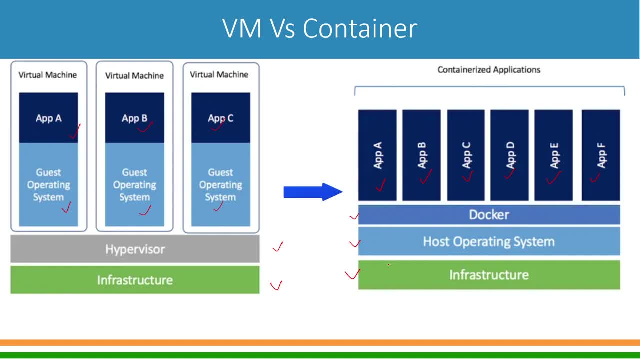 you can kind of allocate resources to each of these separately, so you can have n number of containers and and it becomes so flexible that you can deploy more container, remove container and all so so it becomes more, more and more efficient where in virtual machine environment you are struck up. one more problem which it world faces is that 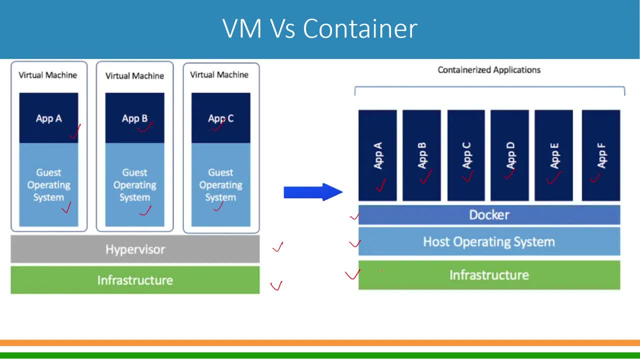 normally all those applications are are developed by some group of developers and and they do this development or on their own machines or developing machines. when it goes to say qa, it may not work sometime. all because so wherever they were working may have a operating system x version, whereas the qa guys may have a y version of that operating system. 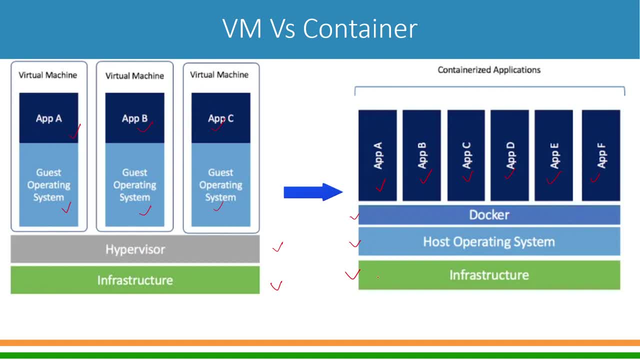 and some of the dependencies would be missing. so sometime the same application which is running on a developer machine will not run on qa machine and even if it has run on qa, it has run on developer machine when you go to production. it may not work all because everywhere they have their own. 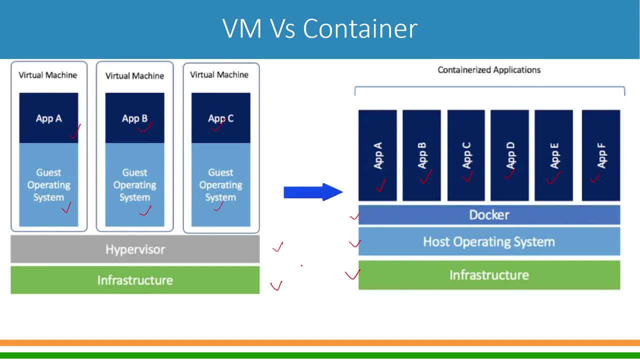 operating system which may have certain uh its own properties, own libraries etc. but in a container environment all those dependencies are part of the container, very lightweight kind of so. so major kernels are there in the host operating system or dependencies comes under the container itself. so it becomes more and more flexible and easy to deploy a. 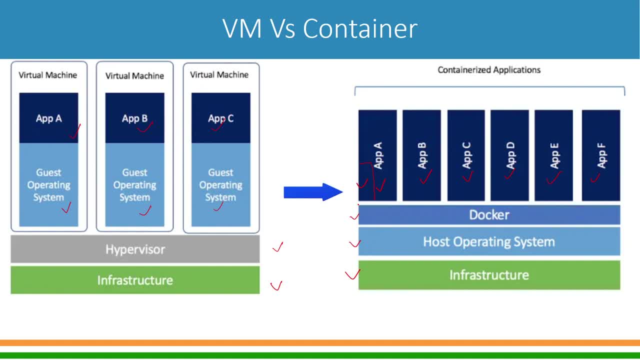 container. so nowadays, if i have to give example, your netflix run on container, google run on google, systems run on container, all big setup. even uida adhar is adopting container environment from last two, three years and everyone in the industry it world are moving towards this. 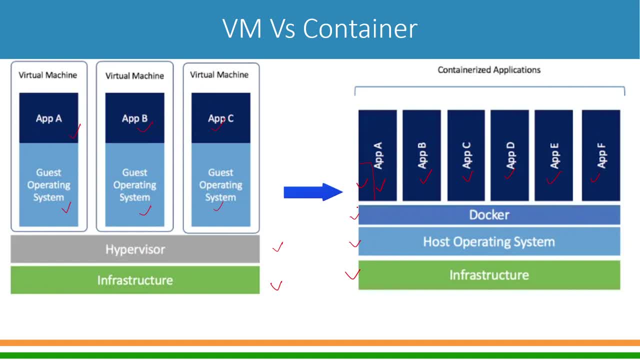 particular environment being being a very, very flexible environment. so i think a few more questions have come, so i'll read that question and try to answer. so one question is from ravindraji: is that: is network visualization possible across different operators or it is a private to one particular operators? and the second question, from ramana sir, is will docker. 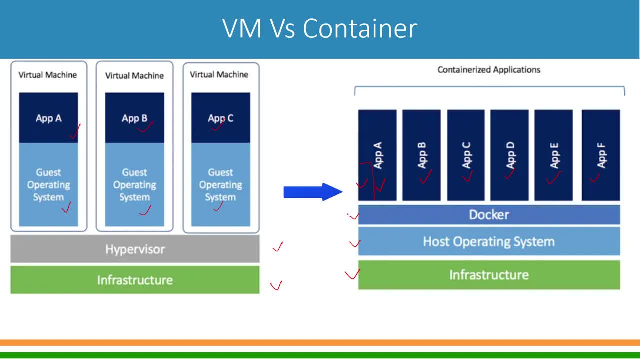 will play hv and uh gos. so if you can elaborate your question, so i i'll answer. in the meantime, i'll answer the window question that you answered. your question is, yes, virtualization. when i have done virtualization, i have also shared a document. if we read, it gives that. so whenever you have an 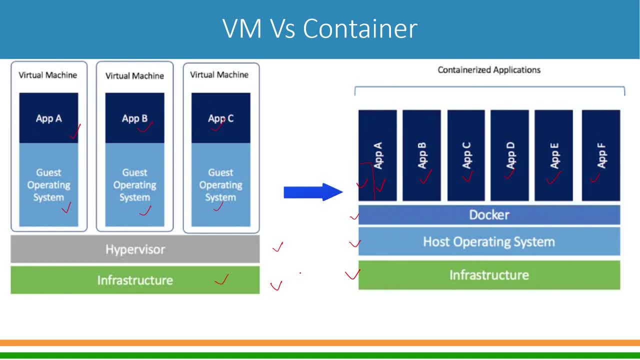 infrastructure virtualized. that is called nfvi and you can have multiple nfvi, so we call it nfvi pop and your some of the network function can be in nfbi pop one. some of the network function can be with nfvi pop 2 and so on. right, so it is possible that some of the network function is is one cloud. 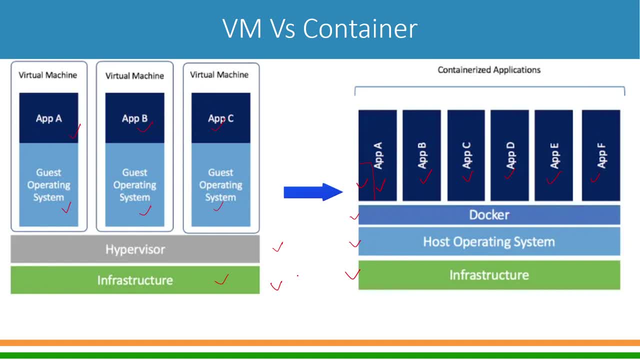 some of that to function in other cloud, whether that cloud is owned by one operator, more than one operator or third party like microsoft, azure, google cloud or even your amazon web services. those all mix and match would be possible in a nfb environment. now the next question, uh. 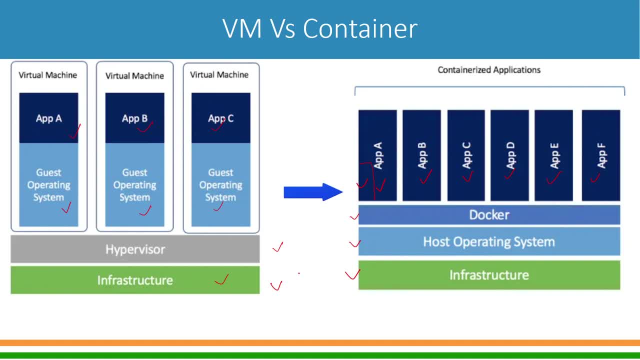 ramana, sir had said that will docker will play hypervisor and guest os. no, just see, the docker is just for containerizing your application, right? so operating system is part of your. it's a host operating system. On top of that, your applications are coming and your applications are having very, very 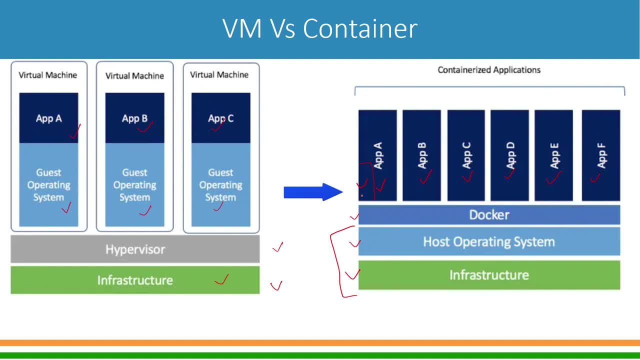 lightweight OS, you can say in the sense, only the dependencies part, I mean the core kernels- are used from the host operating system wherein VMs, every VM, is kind of having a operating system. So in a container environment there is no virtual machine concept, it is directly on. 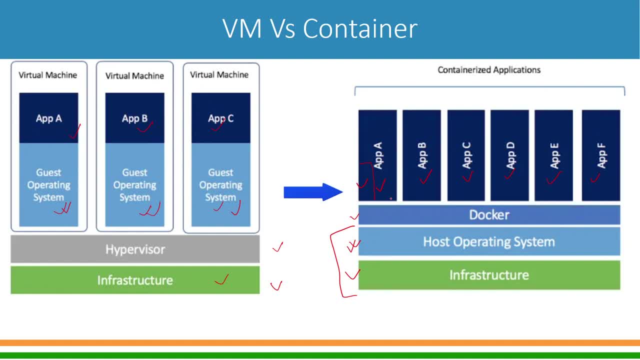 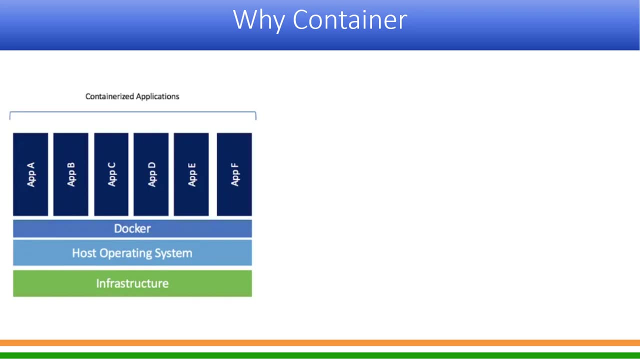 the infrastructure it is running and certain resources are allocated. Yes, Kiran has already answered that docker provides the environment. that is a right answer. Okay, so I think I have already discussed that- why container compared to virtual machines? Let me say that even today, a lot of IT installations are on virtual machines, so I am not kind. 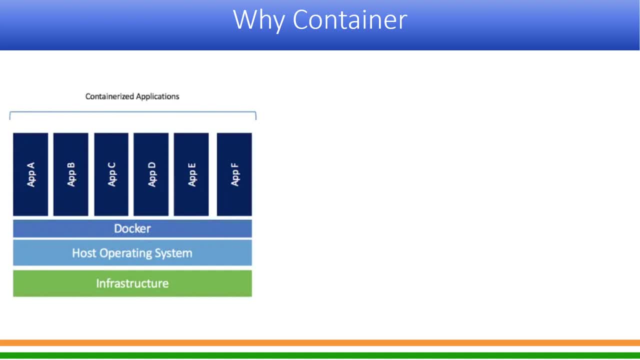 of saying that those are not Not effective. but nowadays all applications are being deployed on the container. even the OEMs, the major OEMs of telecom service providers, have come out with the container environment. So, going forward, everyone is moving towards that. 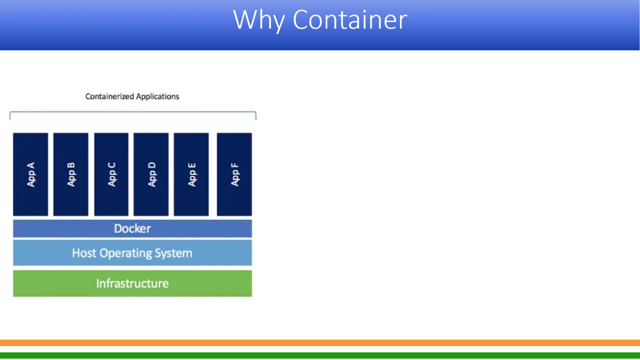 So everyone who is running application on a virtual machine today will have a roadmap to shift to the container environment. So why container? All because we are able to use the resources more efficiently. Okay, In the sense that, since container are light and you can allocate resources anytime you. 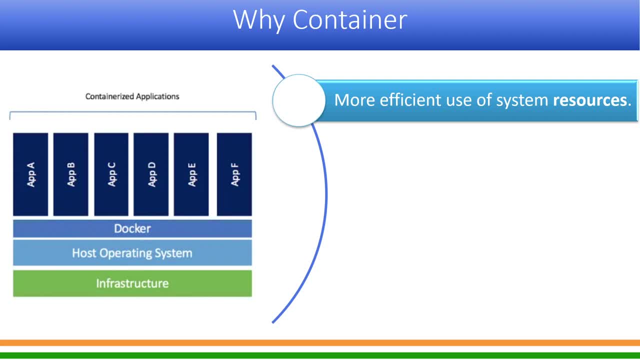 can modify those containers, I mean change those containers, or more than one instances can be deployed. It is very, very configurable, So resources are used very, very efficient way and the deployment is very, very faster. So it is a you can automate your deployment if you have a container environment, because 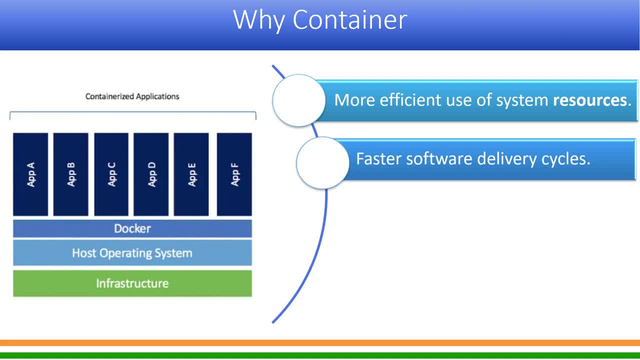 once you have tested A container in a developer machine, you can just deploy through a script. there are a script in the market which will be used to deploy and it becomes very, very smooth. So every small, small patch you can deploy, keep deploying, right. 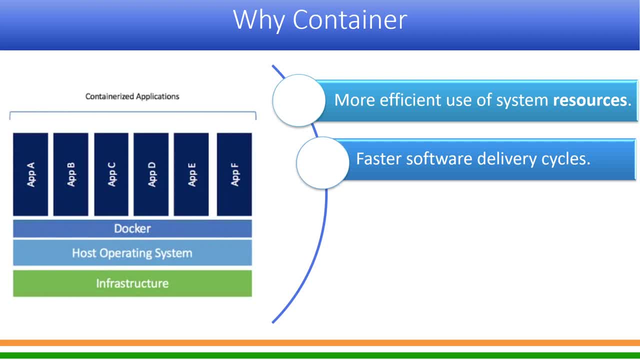 So you did not wait for a complete system to get developed and then deploy the way other versions are deployed. You can keep improving your system and keep deploying, and you can also do a environment wherein you can deploy the entire system. You can deploy the entire system. 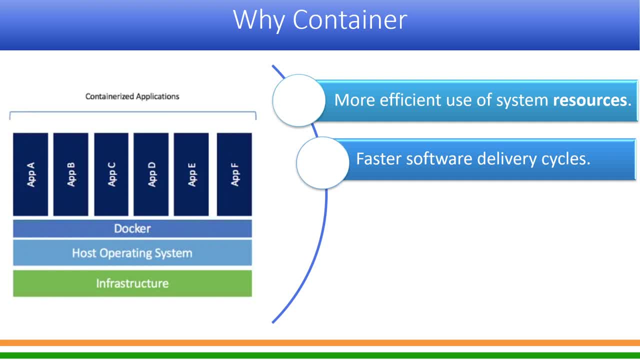 You can deploy the entire system When you deploy a new piece of software. for example, you have created a new version of AMF, So not necessarily you have to replace all. just put in one instance, see how traffic is going on. 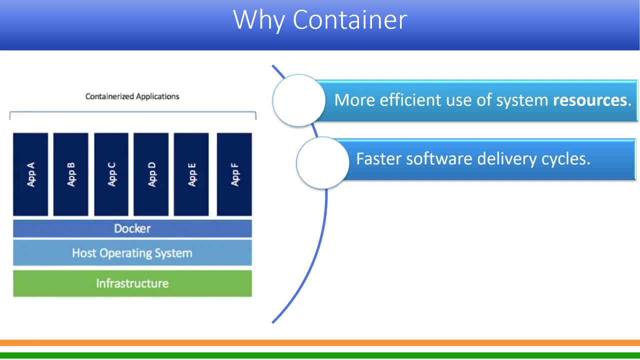 If it is working fine, then you give more traffic. If it is stable, then it replace all other AMF with the new version of AMF. So a lot of agility comes into deployment with this kind of deployment on NFB. Thank you. 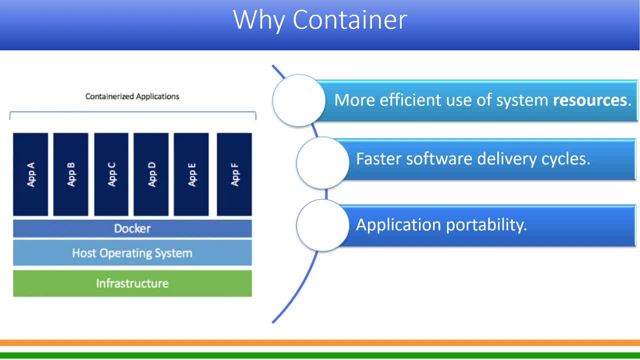 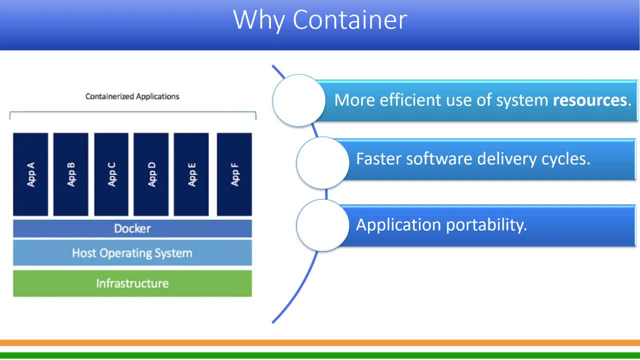 Thank you too, Thank you, Thank you, Thank you. Please come on so we can do stuff and do programming saying that you are not using about. Thank you, sir, Thank you. So we are going to do any other files and IP rules or Ignore these files. 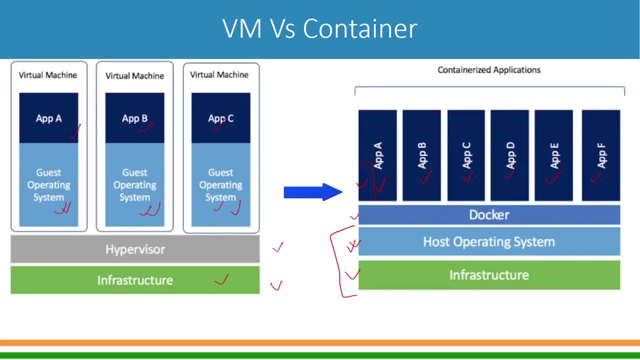 Anything you want to say, your mark and Katin would be happy to take it. Thank you, Thank you so much. Thank you. Thank you. Thanks, любим and Sab forte. so a So here we cannot creating what Okay? 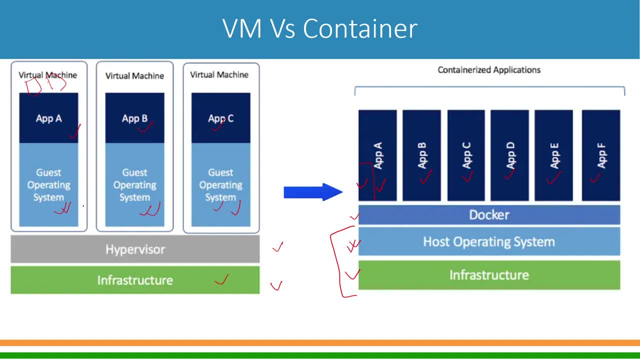 Once you create a virtual machine, so normally it is running a every virtual machine in running a kind of a thick operating system. So it takes your compute, takes your memory, whereas here you have only one operating system, that is host operating system, And these containers are just having the dependencies related to that applications, nothing else. 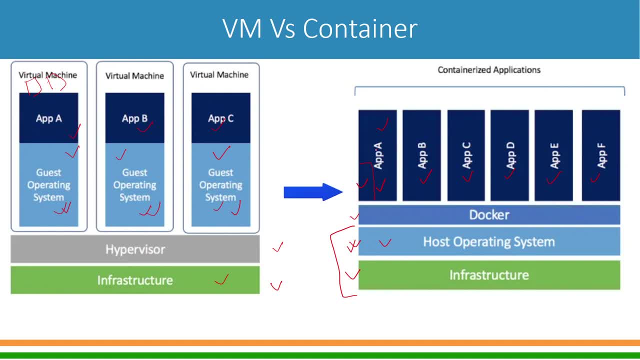 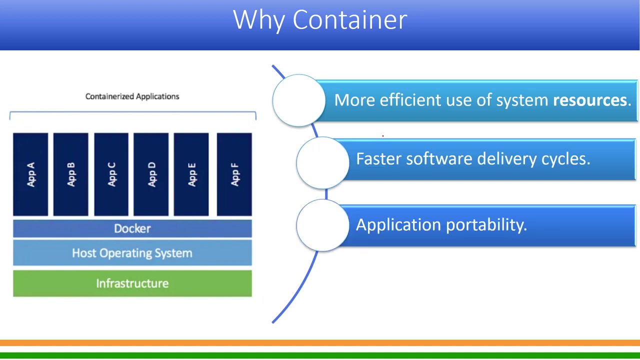 So it becomes very, very thin and kind of a efficient. yeah, these are apps in mobile only, but mobiles are not container environment today. yeah, analogy, yeah, you can say that yes, Okay, so application portability is important aspect that if you have a container, no, so 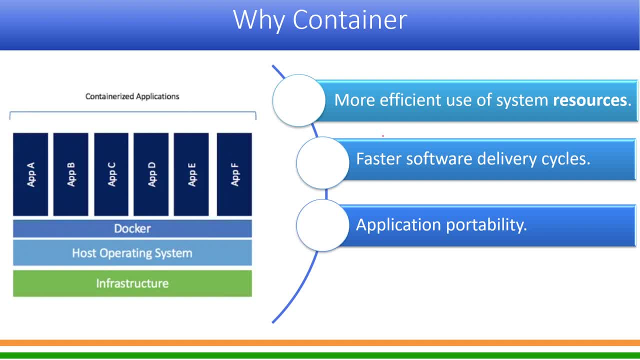 you can share anywhere, you can deploy anywhere. Well, let's say, it's a very, very portable application. it becomes right. And then this enables a micro service architecture, in the sense that, since you can create container application for each and every small thing, for example- I'll give you one example. 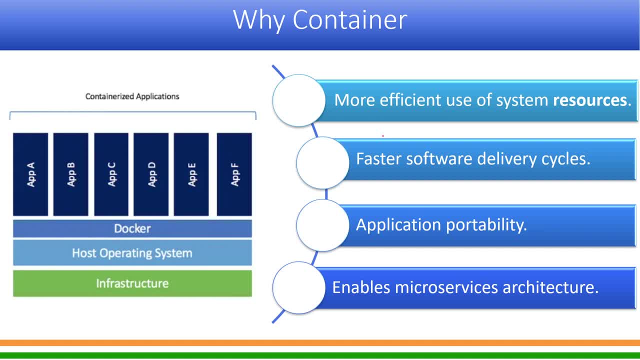 To realize. those who are in IT world already know, but those are new. I just explained that. suppose you, you, you go to some website and then you try to realize a container application. you log in, right. So when you try to log in, you give user ID and password and then then it OTP comes. 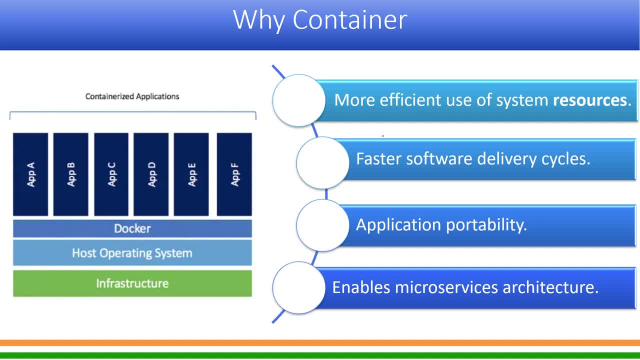 and then you put in the OTP right And then perhaps you enter your demographic right, So whatever. so one way of deploying such application is a monolithic application, that in the background, in the server side, you have one application which is handling all. 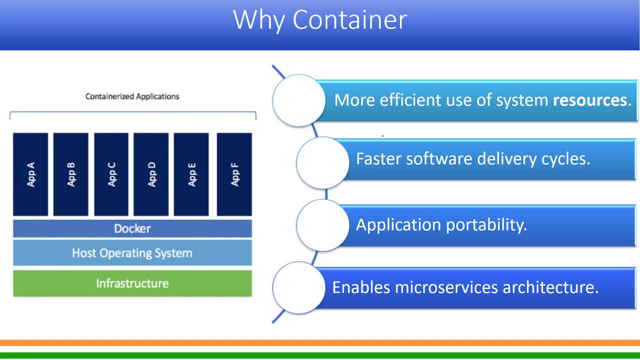 these things. Other way is to create a micro service For each and every element. for example, generation of OTP can be one micro service right, And that application, the front end, will call that application wherever there is a requirement to generate an OTP. 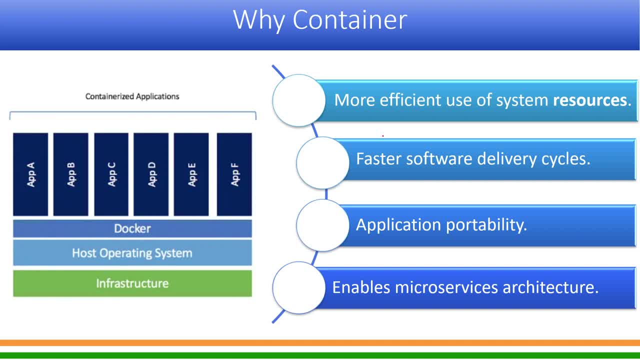 Now taking the OTP entry from the user and validating could be the another service. right User ID and password management part can be the next micro service. entering of demographic can be Next micro service. If you have a validation of those demographic field, the validation can be made a standard. 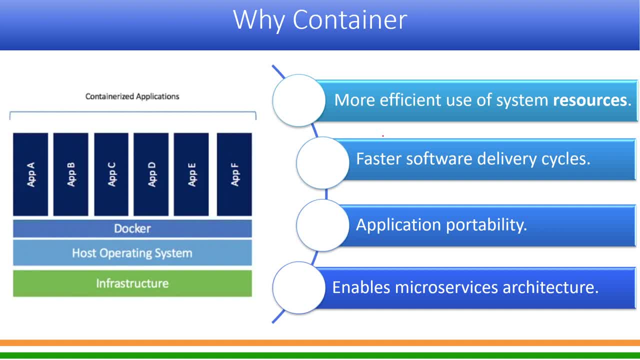 can be made a micro service. So what is the use of advantage of micro service? You need not create those services again and again. suppose you create a next application where again you require an OTP. you don't need to write a code for OTP generation because 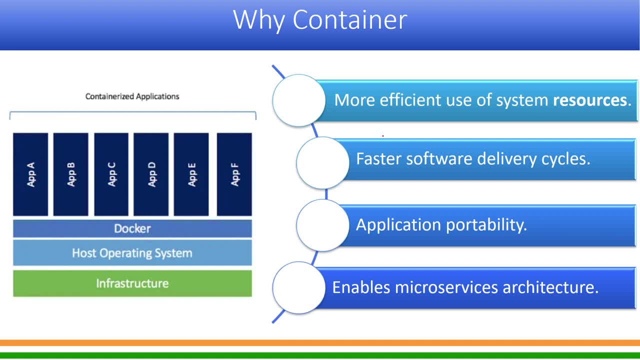 you already have a micro service, just call that micro service and that is available. So that is the advantage of micro service. So here also. So in the case of a 5G, every network function will be a micro service. Not only that, every network function can be set up for five micro service right. 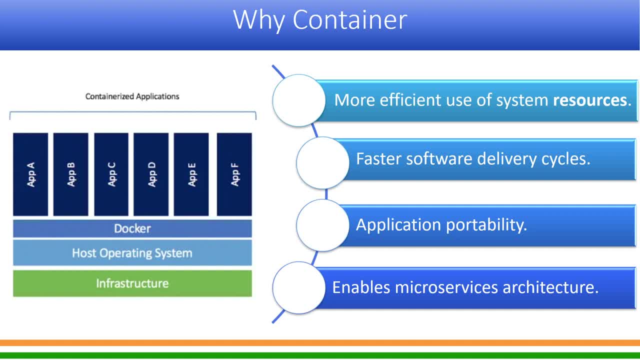 It's not necessarily that the entire network function is only one micro service. it can be set up multiple micro service also, So so the container environment is more suitable for micro service architecture. I'm not saying that microservice cannot be deployed on virtual machine. 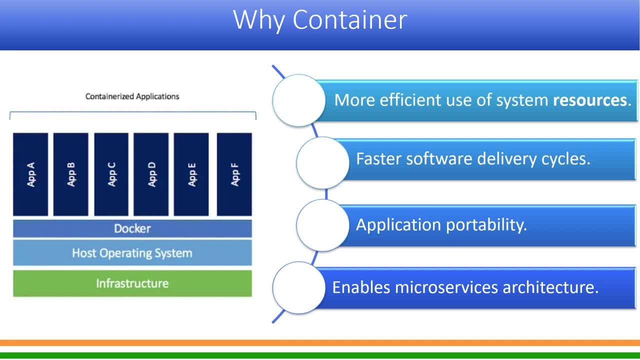 Yes, can be, but it becomes more and more useful and manageable in a container environment. so there is a question that how many containers can be created in one vm or in one infrastructure? let me take that question. so answer is there is no limit, as such limit will be your traffic, for example, if you have a limited infrastructure, compute and memory. 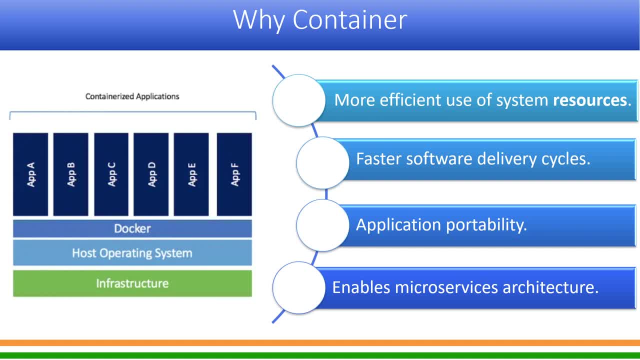 and if you deploy too many containers, so there will be congestion, there will be problem. so it depends upon and, and then, uh, you have to scale it up right, so you have to suppose you are running out of memory. then you can insert more memory into infrastructure if 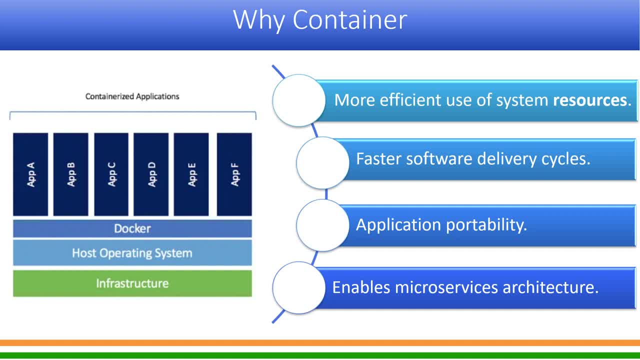 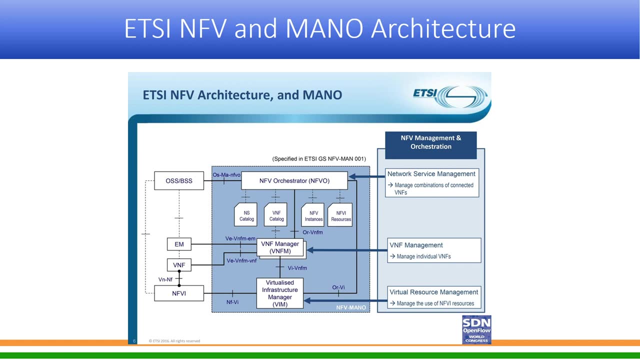 you're running out of compute, you insert more server blades into it, so there is theoretical limit. of container will not be there. it's all manageability, right? okay, so this is archi. this is the architecture diagram of nfv and mano by its. it is same. 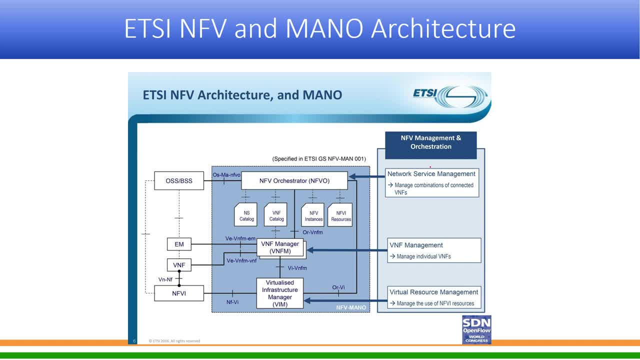 which i discussed. so it has got multiple layer. i'll just read. so the lowest one is called nfvi, so that is network function virtualization infrastructure and on to this. so here you actually manage the virtual resources, all those physical hardware, server memory. those management becomes and you create a virtual infrastructure. and then you create a virtual infrastructure. 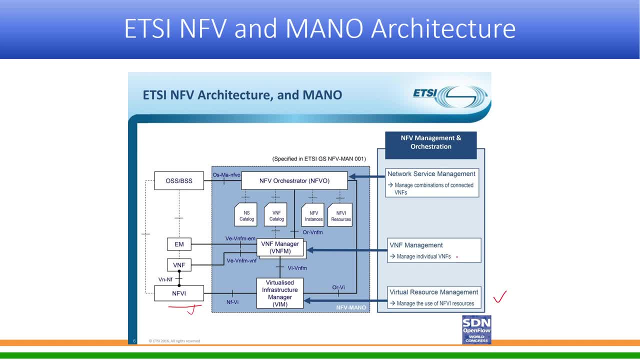 create an environment, the virtual environment. on top of that you have vnf, so you will have vnf management, your so you will have kind of a vnf manager where these vnf will be managed, and you also have element managers and top of that, on top of that, you have a network service management. 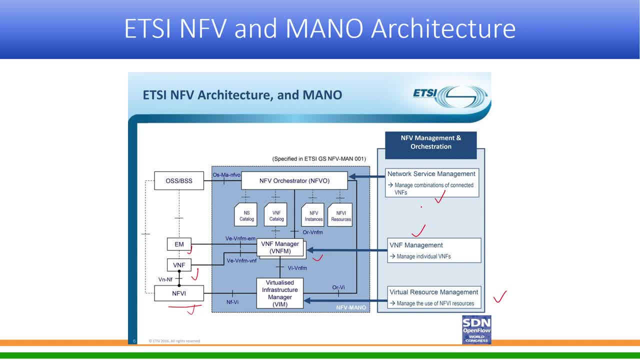 which vnf to create, which we have to delete, which we have to modify. so that is called orchestration also. and then you connect your oss and bss. so that is broad architecture given by uh hc. on right side whatever you saw is kind of nfb management and operation and on the left side you have all those. 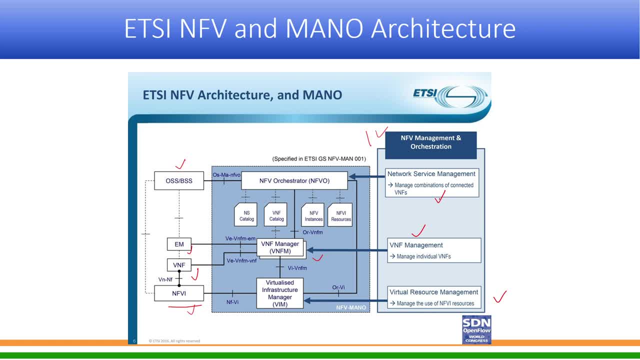 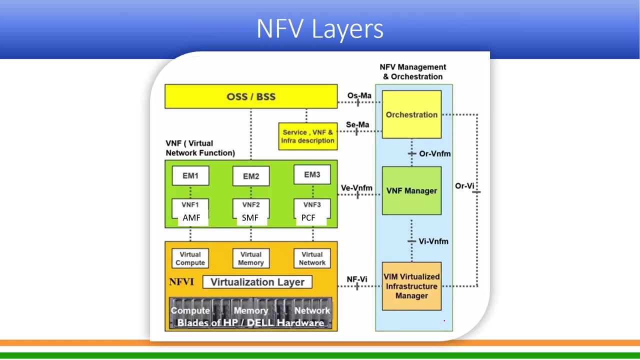 elements. so this picture i have taken from one of their webinar which is freely available on to onto their website, which is they had done it for sdn open flow world congress. it's a very good picture and this picture is also there in their specific classification document which i have shared. so let me explain, uh, the three layers which 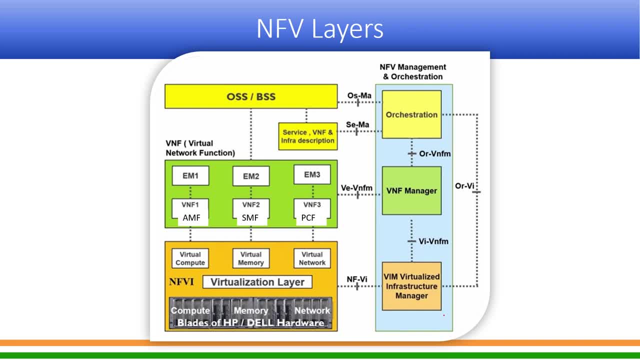 i talked about in a slightly colorful picture, so, uh, i'll just explain. so. so what are three layers? the first layer is your virtualized layer, that is, virtualization layer, we call it so. in this virtualization layer you have physical compute, your blade servers, physical memory and the 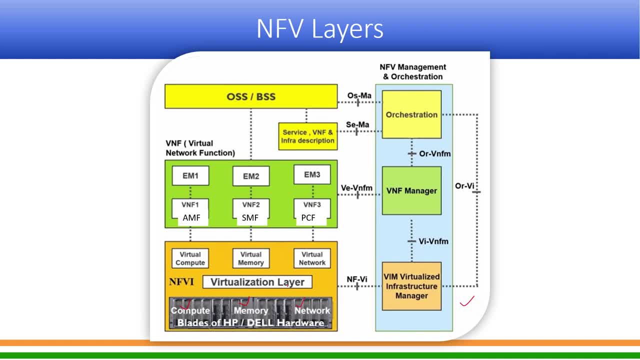 network, and you are able to virtualize using any virtualization environment, hyper hypervisor, or you can containerize in that sense. so, finally, you create virtual compute, virtual memory and virtual network on top of that. so that is the layer one. the second layer is the vnf itself. onto the virtualized environment you can create virtual network function, one that may be a. 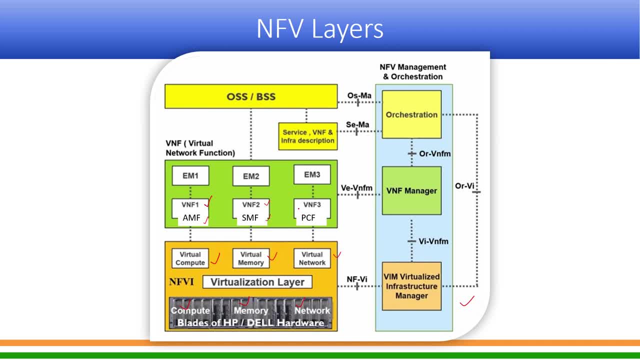 mf. example: vnf2 can be your smf, vnf3 could be your pcf and so on, and there will be element manager. these specific vnf can be managed through the element manager and the overall management of vnf will be done by vnf manager, which is part of the manual. and then, finally, the orchestration. 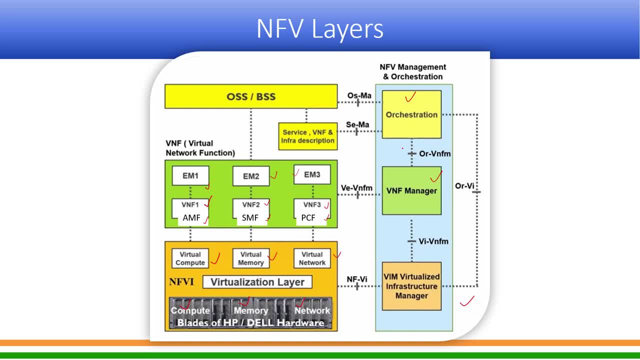 i mean, all those management will be done using the orchestration. so, three layers- you you saw this- this: layer 1, layer 2 and layer 3.. We will discuss these one by one. So the first of all, virtual virtualized infrastructure manager, this one, the lower part, the lower part which I already 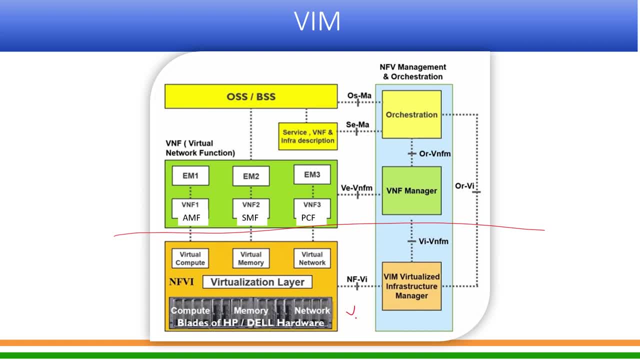 explained that the physical hardware is virtualized using any software, VMware or any hypervisor to create a virtual compute, virtual memory and virtual network. So that is our virtualized infrastructure manager, which does of course, the command come from the top which manages these two functions. If you look at VNF managers, that this one. so basically the function. 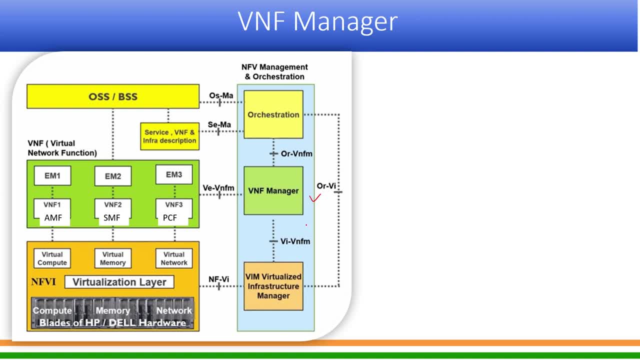 of VNF virtual network function manager is the life cycle management of these VNF life cycle management. when I say life cycle suppose a new AMF is to be created, right. So those will be done by the VNF manager: creation of a new network function or creation of. 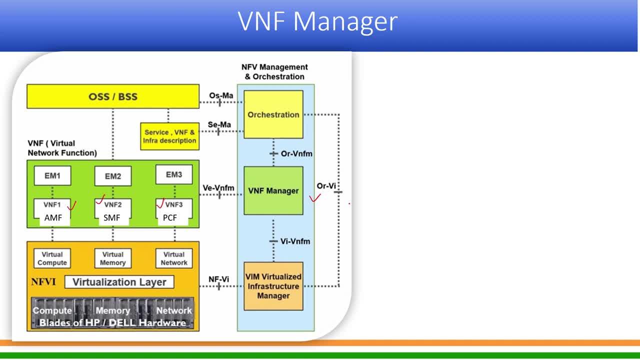 a modification of a network function, or suppose some network function is to be deleted. So all these will be done, done by this VNF manager, this part, the green part we are talking about, So the life cycle management of the VNF. so it includes creation of a network, modification of 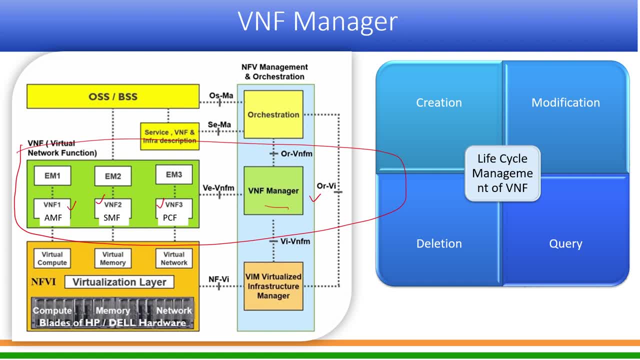 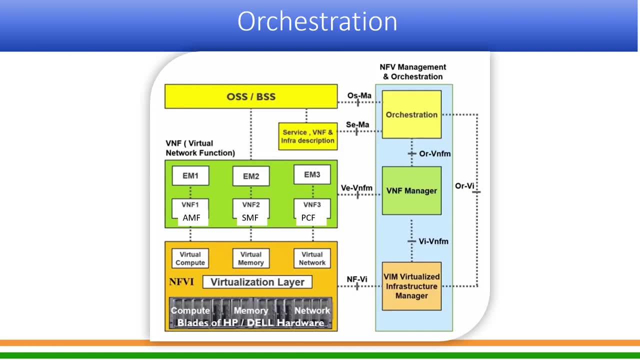 deletion if required and also if you want to query or do something. So the VNF manager comes into the picture right and the top part is the orchestration. all those orchestrations are being done by the top part. which kind of a brain in the sense that to. 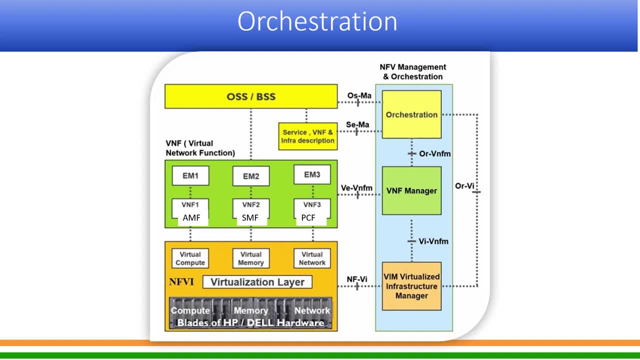 manage the entire infrastructure. So once we have virtualized the network, the integration of all the network functions can be done with a simple call to the, the VNF manager, for example. We want to create a big variety of network functions and we can create the kind of network functions using the. 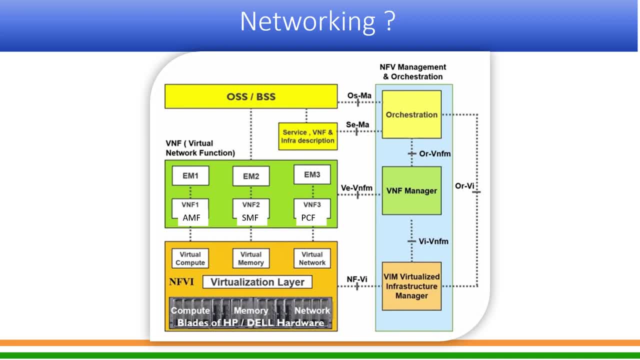 would be possible. but all these network functions, since i said that there can be multiple nfvi, some and nfb would be at one place, some nfb would be at other place, and then it's a big network spread across the country or a region. so those are connected, so there is a networking involved, right? 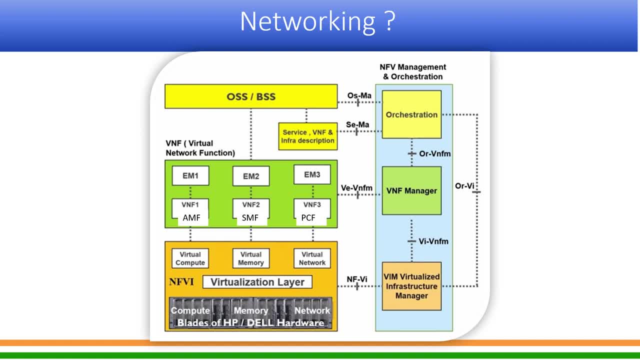 so suppose i create a network function like amf, right? so amf will have a specific ip address, a specific fqdn fully qualified domain name, unless those items are known to the entire network, although you have created the network function. but it may not be able to be utilized. so we again have a bottleneck on networking right. 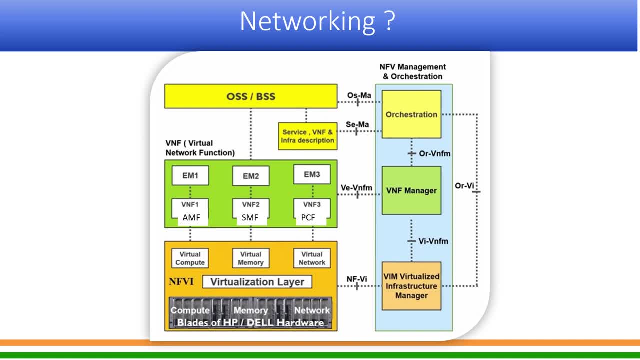 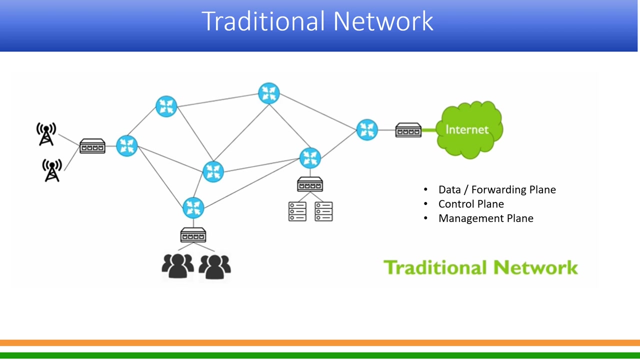 so unless the networking is also kind of advertised- the network address or the new network function address- it doesn't come into utilization quickly if you have to connect to the network outside the particular nfbi pop. so the question is how to manage network. so so traditional network, if you look, it's a kind of router and switches are spread all across which connects. 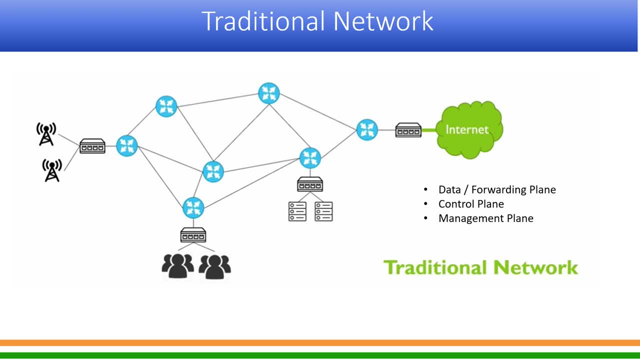 your infrastructure, all your data center where network functions are deployed. right so this? in this picture you see routers and switches installed at various locations. right so, but in such traditional routers what happens is that that data plane, where your data forwarding takes place in these routers, and also management of these routers are here itself, in these boxes itself. so that means 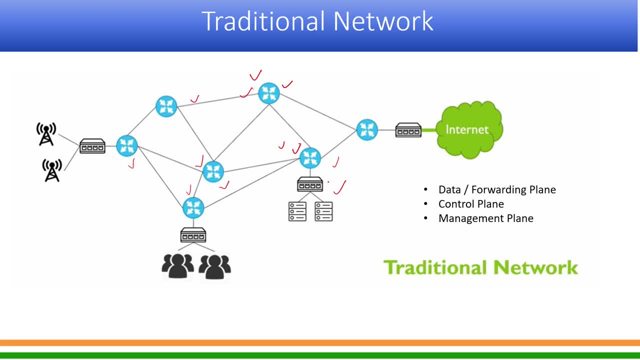 that someone has to login remotely to these boxes and every time they have to configure, whenever a new uh network element is introduced, that the ip addresses are changing. whatever you do, you have to again, so that becomes a tedious work. so I got with NFB. I am not able to actually- I mean take the advantage of that. 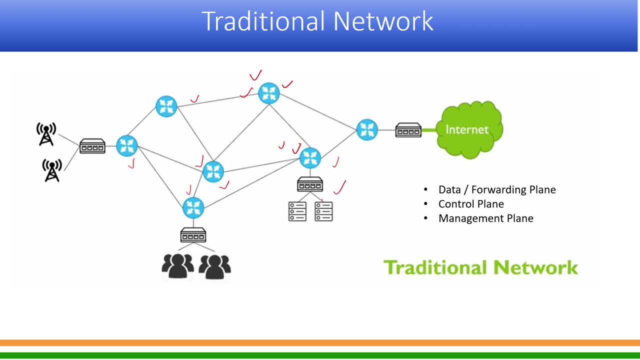 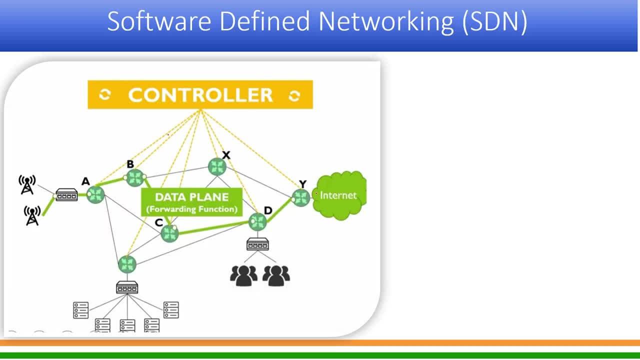 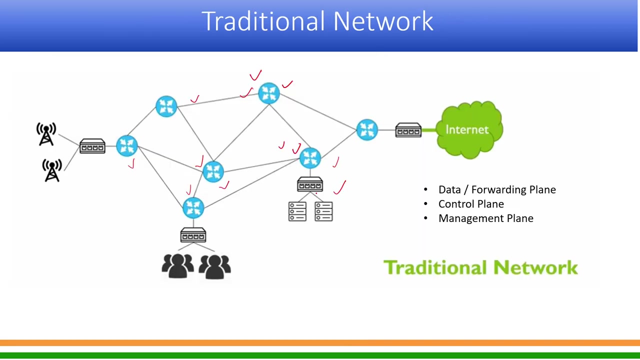 So that is a problem with the current networking. So here comes the concept of SDN, Software Defined Networking. So many a time this term gets confused by many of us that what is software defined networking? It's nothing but what is done in the previous case, just like when we talked about NFB or 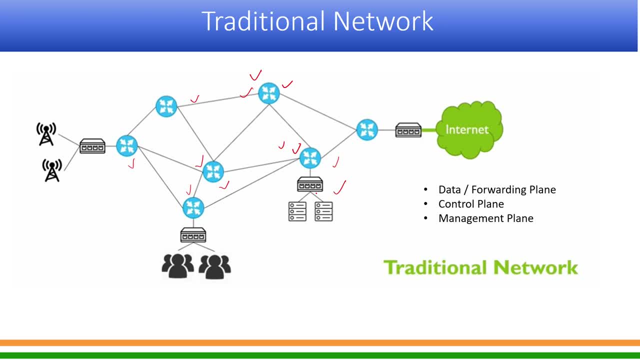 talked about service based architecture of 5G, we said that we are separating out user plane and control plane. That means we are separating the user plane where traffic flows, with the control plane which manages. So here also we will kind of separate out the management plane from these routers and 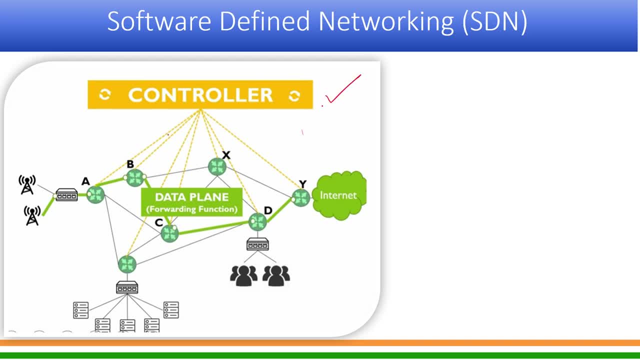 make it centralized. So basically, So the control part comes at a central location and at respective locations you only have a data plane or the forwarding function. So now the entire network of, I mean where all those 5G functions are connected, or for 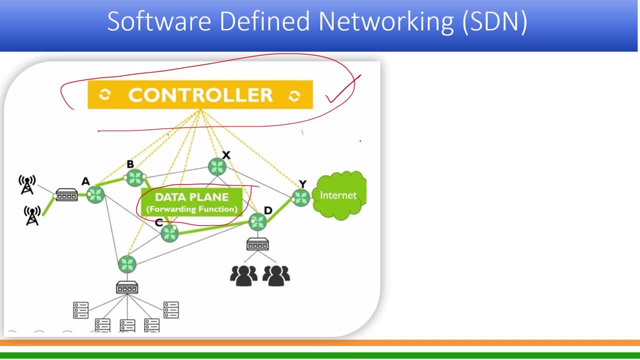 that matter, any other IT systems are connected, it becomes easier. So, along with NFB, you can also program these aspects centrally, and then it becomes very, very smooth. So this is a basic thing. This is a basic concept of software defined networking, which our friend from IT field 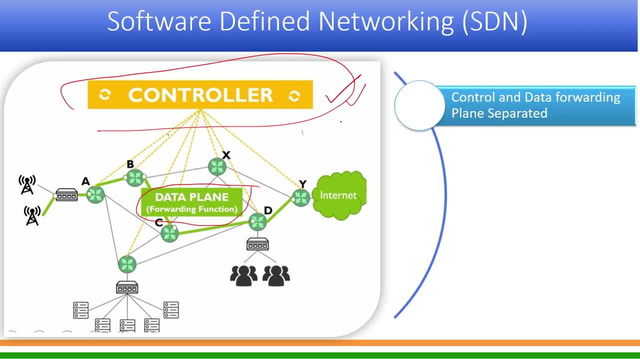 would know better. So basically what we are trying to do in SDN is that control and data forwarding plane we are separating out so that we can manage centrally. So entire management is centralized. So that makes our networking and IP routing very, very flexible. 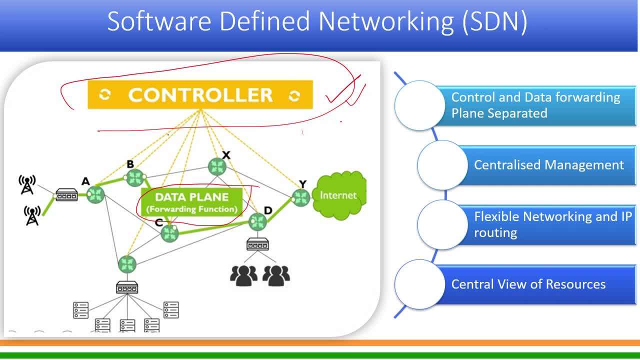 And then you can control or view all your resources centrally. So that makes our networking and IP routing very, very flexible. And then you can control or view all your resources centrally. So that makes our networking and IP routing very, very flexible. And then you can control or view all your resources centrally. 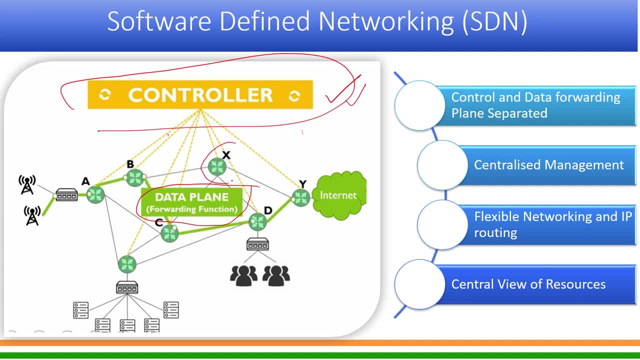 Whether, for example, in this example, suppose this router goes down So your central system can configure your traffic to go from alternate routes and all Automatically either can be programmed or, if something new is happening, that can be done centrally instead of requirement of logging into the respective switches or router. and 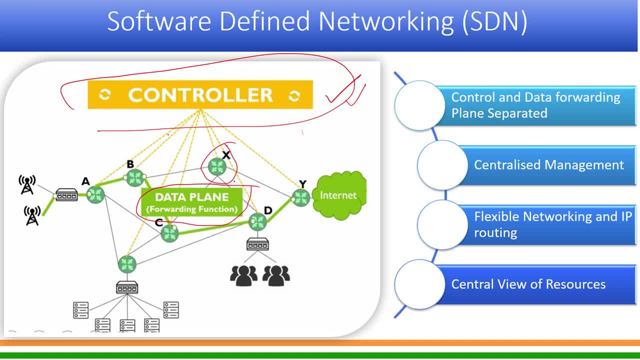 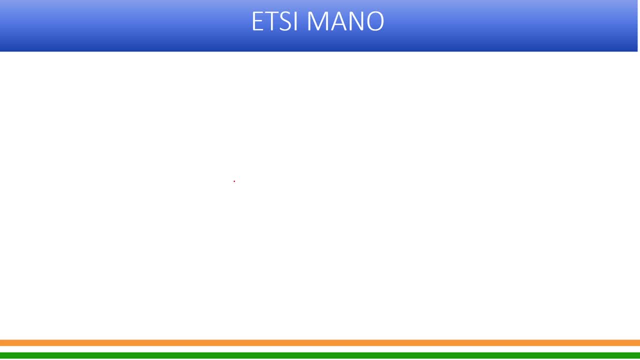 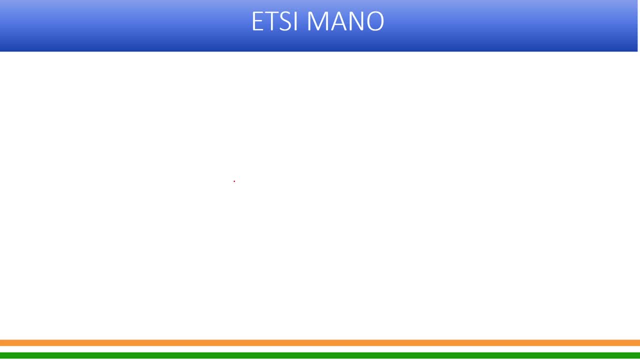 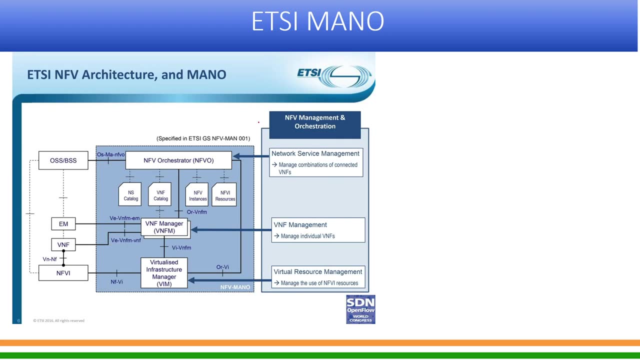 So now I talked about management and orchestration. That is also a piece of software. So what it sees doing is that the ITC is developing the Meno software, open source Mano. they call it open source Meno. So the Meno part, the right side part, if you look at this particular aspect, I mean 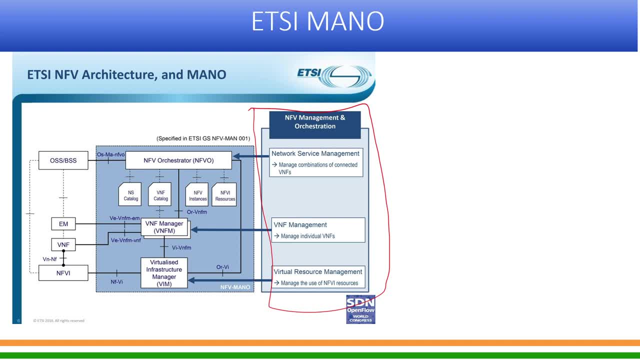 anybody can develop this software, but they have come out when open source manual. So, and they have been working on it. recently They released a list of stuff And, but this particular is a version called OSM release 10. that is, open source- MANO release 10.. So last year, when I was 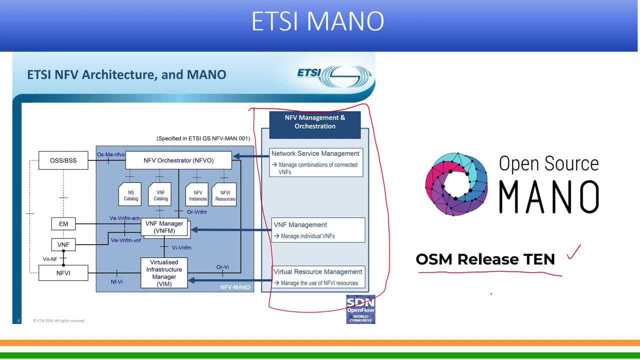 teaching about this. it was release 7. So they have improved upon this version- and this is publicly available to all operators- that if they want to deploy NFB, they can actually choose to use ITC MANO, which is an open source. So that is one of the advantage of going towards the NFB, which 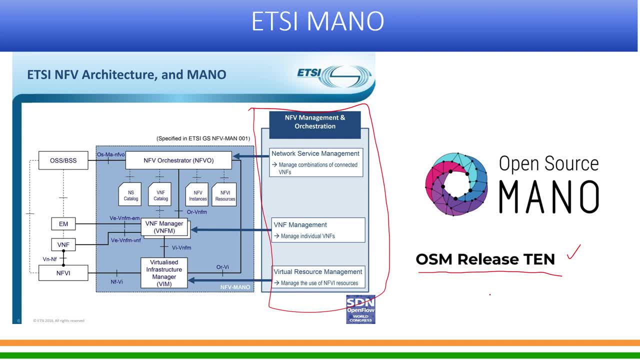 becomes a kind of enabling factor for open source. We have been hearing about open source, RAN and all, and also the 5G core on an open source environment. So this is one of the kind of initiative which standard making body like ITC is undergoing. So and the 3GPP standard of 5G. 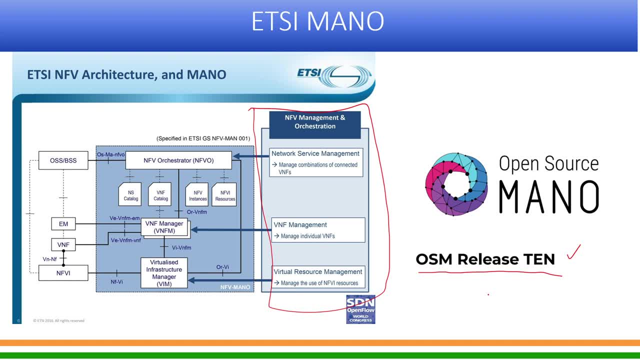 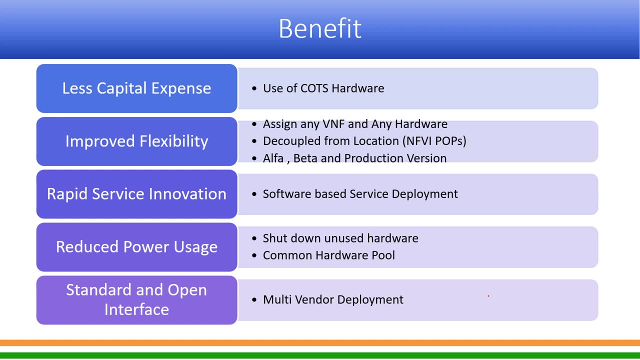 is such that you can actually adopt ITC NFB and ITC MANO. Those are kind of complementary to each other. Okay, so let us finally- I mean, revise the benefit of MANO. So basically, we can use COTS hardware commercially of the self hardware We are not required to get. 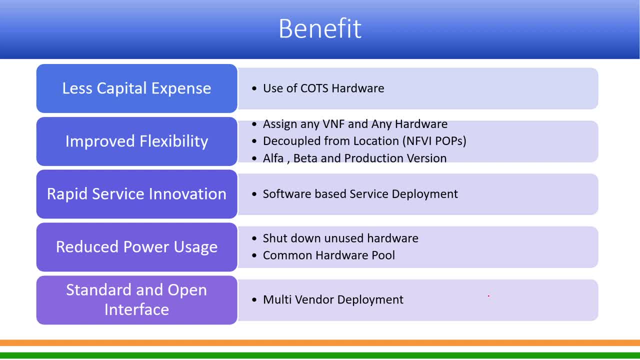 ourselves logged with a particular server vendor or particular OEMs of the telecom infrastructure. The flexibility gets improved, all because I can assign any virtual network function with any hardware. and location is also not now important because I can have multiple NFBI POPs which is decoupled from the location. So we are also disaggregating the location and then you can. 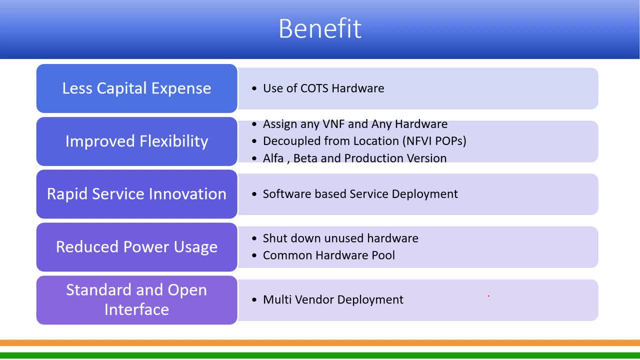 have an alpha production version, beta production version and finally production version. When I say alpha beta, that means when you come out with a new version of software network function you deploy to alpha set of customers, maybe 500 customers. If it is working well, you move to a larger set of function or in case it is giving trouble, you can always 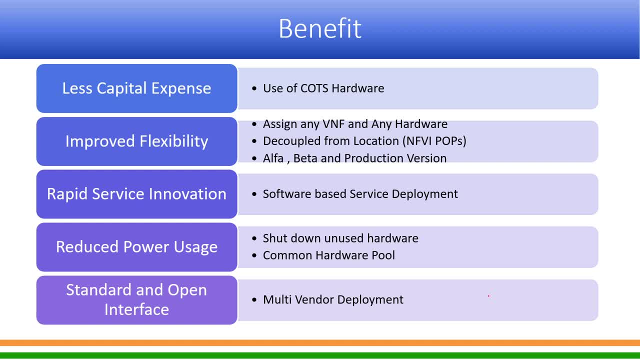 withdraw and improve upon. So it gives you flexibility in in deployment and testing your new software and your service. innovation becomes very, very important. You can deploy your service very important- and the power usage is reduced. As I said, that you can scale down, scale up, 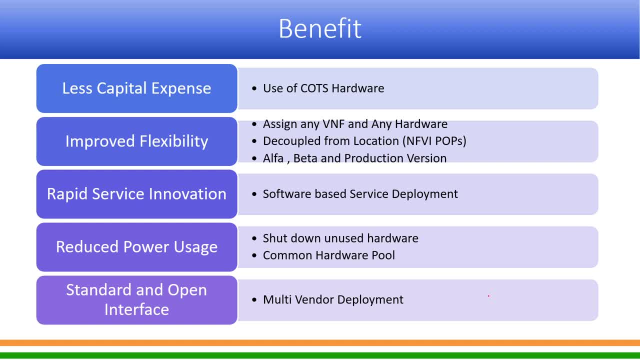 and being a common hardware pool, your power usage is less, and then you can you have a standard and open interface, so it becomes a multi vendor environment. So with this my NFB part is complete. I will be moving to the network slicing portion. So if you have any question I will answer and then 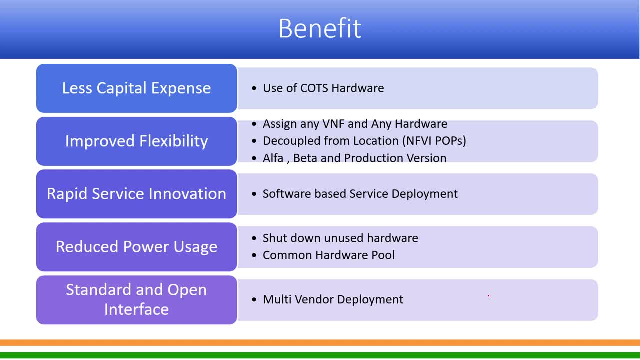 on NFB and we will move towards network slicing. You can write in chat box or open your mic or anyway, whatever you like. or let me ask you whether you are basically whether, where, whether you will be- you are able to understand the concept of NFB at least. 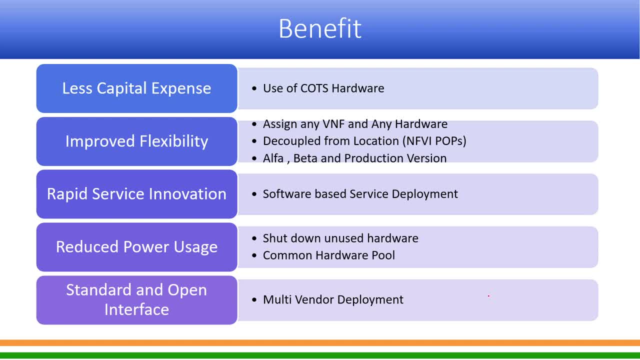 Yeah, So in a virtualized machine environment. so every virtual machine will require its own operating system And normally if you look at operating system, so maybe your- I mean very, very spaces in very, very huge memory- would be required to install a guest operating system, Whereas in a container. 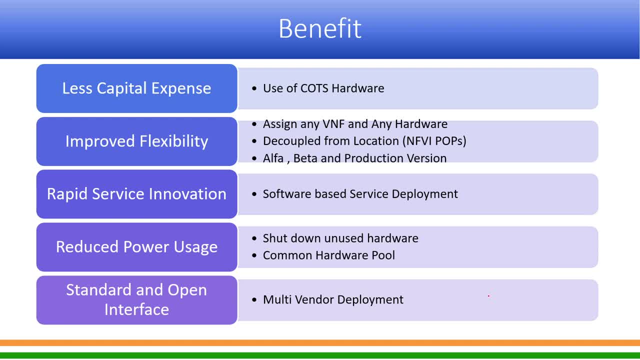 environment. you can install a guest operating system So you can install a guest operating system. You can install a guest operating system So you can have your own container. But if you go that host and you want to install a host, You need to have a host operating system in the container So you can use the host operating system. 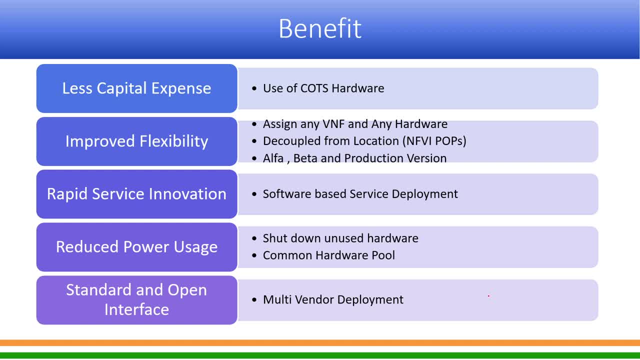 it uses the host operating system and only the dependencies. which is required is part of the container And and deployment of container is such that you can import a container from wherever it has been developed and just deploy, which becomes like a copy paste command. It just becomes like a copy paste command, whereas onto the VM environment you actually 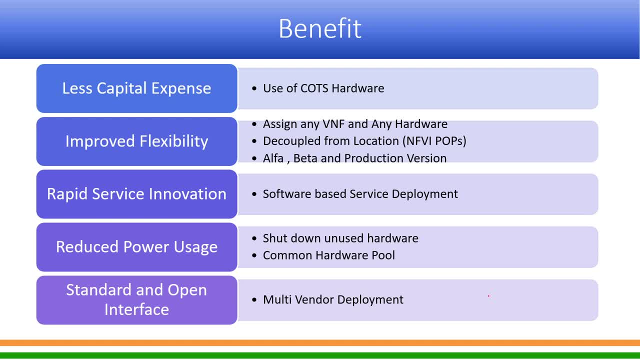 install that particular application and run it and you have to see that it is compatible to the guest operating system of the VM from where it was actually developed on a developer machine or some other vendor machine. So that becomes a challenge. And then number of container you can have on a particular infrastructure. that number 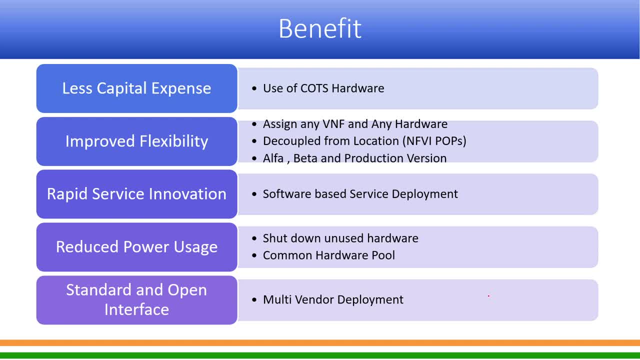 of VM you may not be able to have because every machine would require minimum kind of compute and memory because of the guest operating system, and then on top of that you are applying the applications. I hope I was able to answer yourself. Yeah, yeah, please go ahead, Kiran. 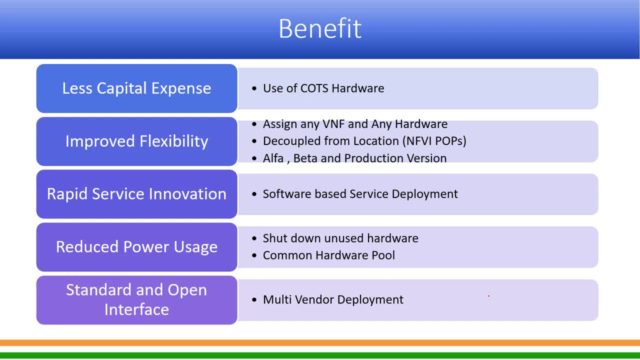 Thank you everyone. Thank you everyone. Thank you, Thanks to all of you. You are right, Kiran. all because I mean you guys are using it. So basically, you can. what you should consider is that the container becomes more flexible in terms of using the resources or even from the perspective of the applications which 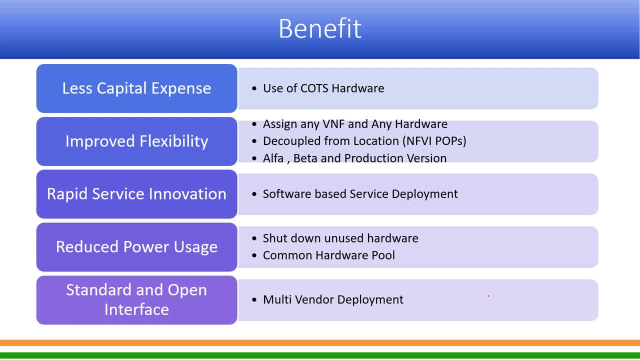 you are making it becomes more flexible to deploy. That is why Google, Netflix, Facebook- everyone has shifted to the container environment. Even in India, many IT systems are using container. So, Kiran, do you have any application running on containers in CDOT? 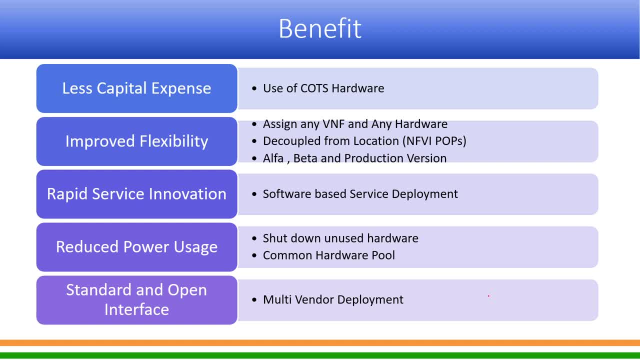 So are you using Docker or some other application for containerization? Kubernetes is for management, Kiran Kubernetes manages ok, ok, ok, the manual part for CDOT is Kubernetes. Kubernetes, I mean, just for the sake of everyone, information. Kubernetes was initially owned. 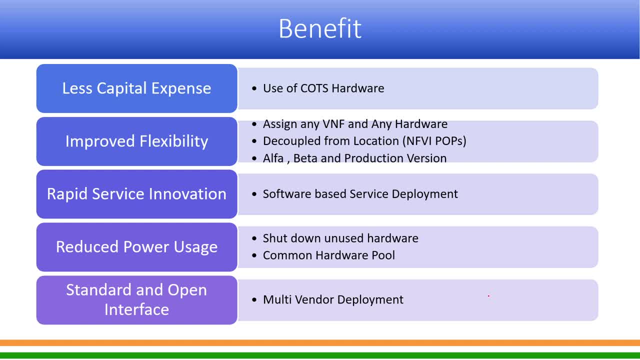 by Google. then they open sourced it. So now it is an open source and anyone can use it. rather now, lot of innovation has gone into Kubernetes once it was made open source, because everyone is contributing. Sandeep sir has some questions, so there is a raised hand, I see. 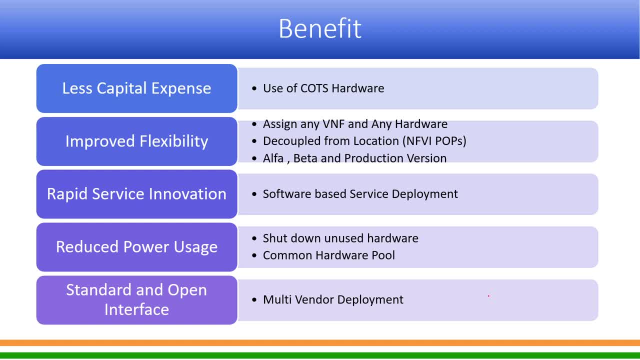 Sorry, do we have a call or something more on the computer in the background? Thank you, Kiran, I have a question for you, So I just wanted to point out something. you know it was a private question, but yeah. 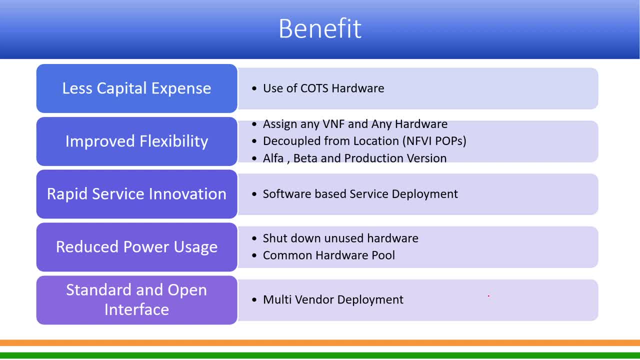 it is a private question. So, yeah, Hi, what is the connection? Hello, Yeah, right, sir. I mean, you are right in that sense. and although we are talking about 5G, this NFB is common to all technologies, sir, all technology. it is not limited to 5G, but 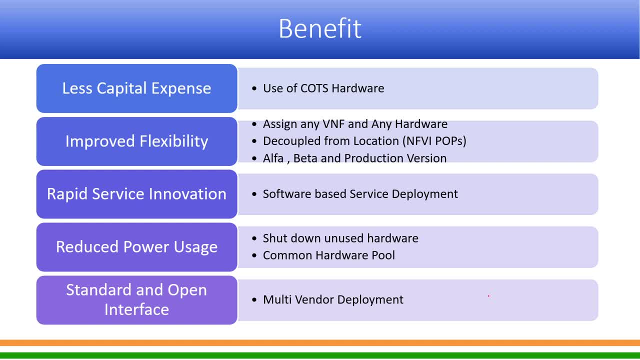 5G is moving towards IT world. that is why we are talking about this virtualization and all. Yes, I mean this. and one more thing which now I want to tell you: that ITC is working on NFB infrastructure from 2013,, 12-13 onwards itself, but now only it is being realized. 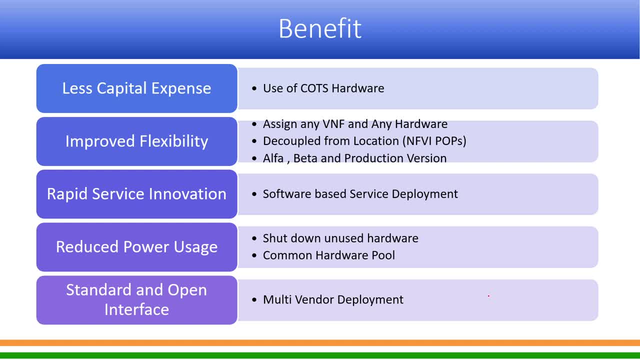 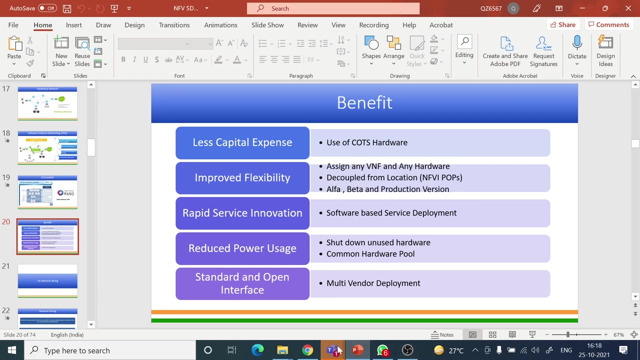 that the telecom infrastructure is actually being virtualized and being deployed on a virtualized infrastructure. so yeah, yeah, Kiran, yeah, yes, Kiran, Yes, yes, you are audible, Kiran. so you are audible. my voice is not coming. let me see. 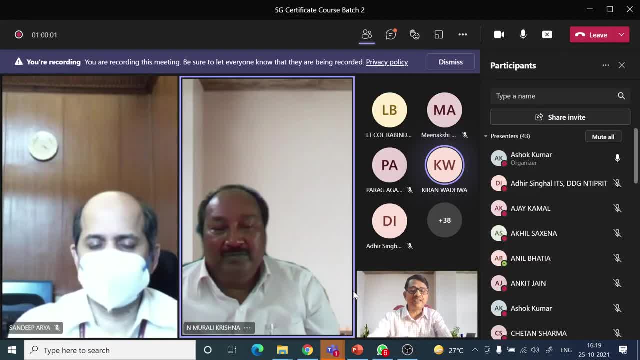 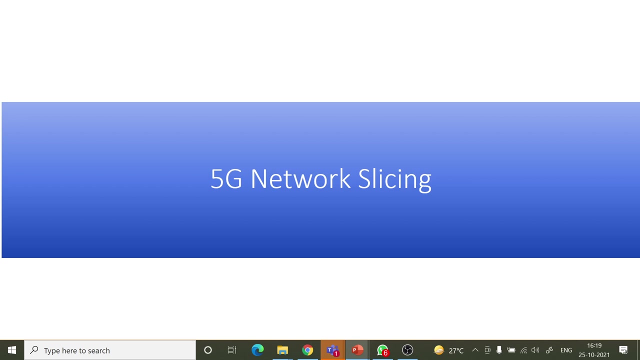 if my so, is my voice coming or my voice is also not coming? can somebody confirm? Is my voice coming? okay, okay, right, so let me proceed further. yeah, okay, So let us talk about 5G network slicing. I think this topic has been covered in many. 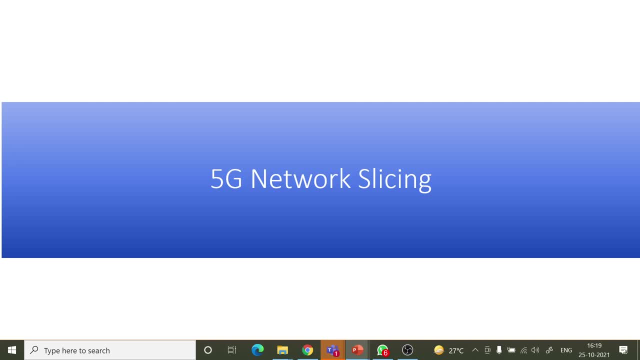 of the sessions, so many of the things would maybe a kind of repeat. but just in the perspective of 5G We have understood NFB and how NFB is important in network slicing. all because the flexibility of deployment, various network function, is the requirement of network slicing. 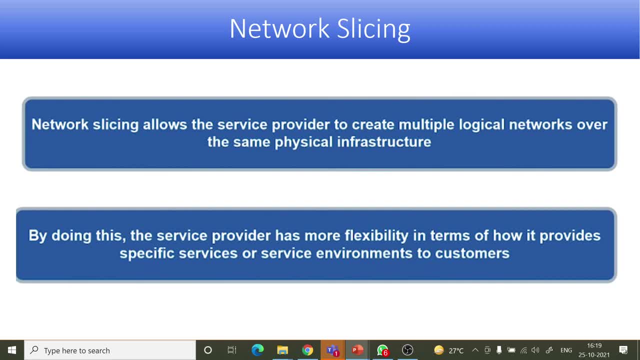 So from the definition perspective, the network slicing allows service provider to create multiple logical network over the same physical infrastructure. So they virtualized kind of a. you can say that they have multiple 5G core, multiple 5G radio perspective. you can understand in that sense. 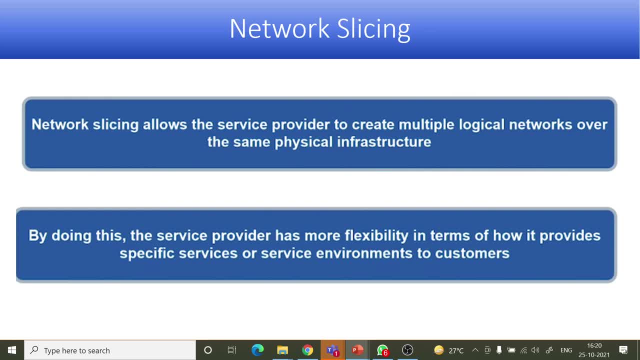 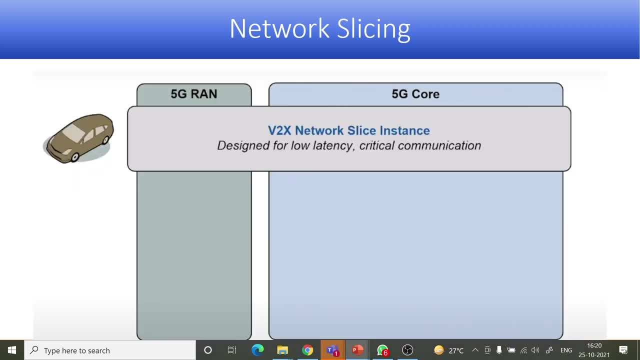 In that sense the provider, service providers will have more flexibility to provide different services or the service environment to their respective customers. So for example, I mean we have seen this kind of picture earlier, that for different services. So here example given is the V2X vehicle to anything connected to the network. 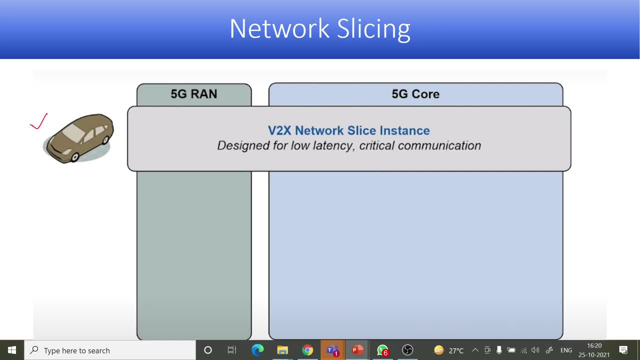 Yes, Yes, Yes, Yes, Yes, Yes, Yes, That is the V2X connectivity which will be one of the major application. is the autonomous car that they can have. a slice instance specifically meant for V2X services, which. 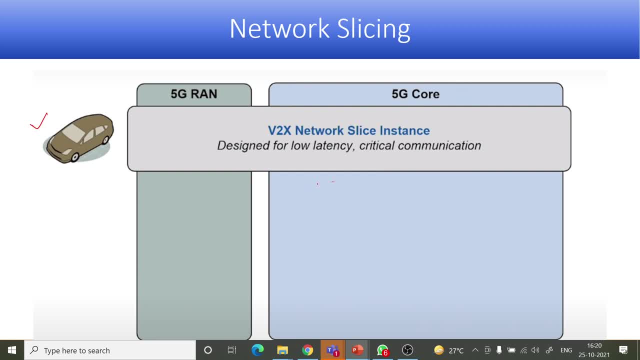 normally requires very, very low latency, very, very low latency, And that also comes under critical communication, that is, URLLC. if you recall, we discussed The second slice. I mean just for example. I will show you the first slice. 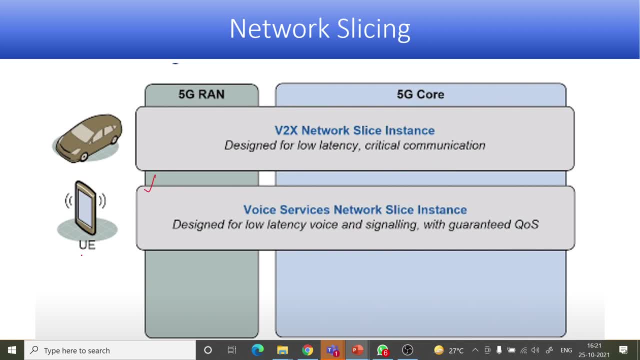 example can be a voice service, As we know that for voice the latency requirement is important and the guaranteed quality of service we had seen the guaranteed QoS will be required and latency in voice and signaling, both would be required. So the second slice example. 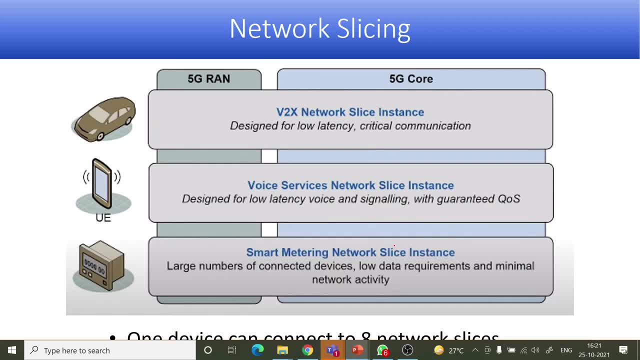 is for voice. There can be third slice, which is, say, a smart metering application. This is one of the IoT kind of application where data requirement is low but it has network activity is low but large number of such devices will get connected and these devices 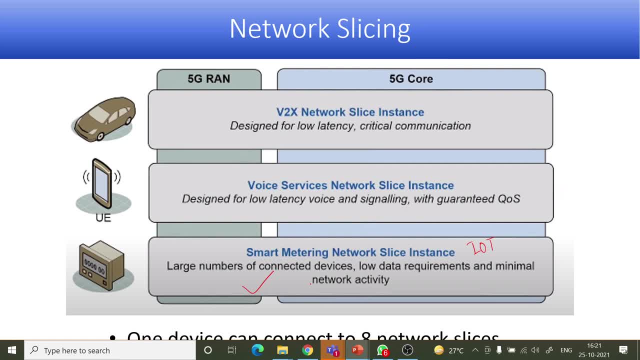 will be installed inside house, basement, etc. So deep coverage would be the requirement. So there can be a specific slice in the 5G, So there can be a global network which will be serving the smart metering application. 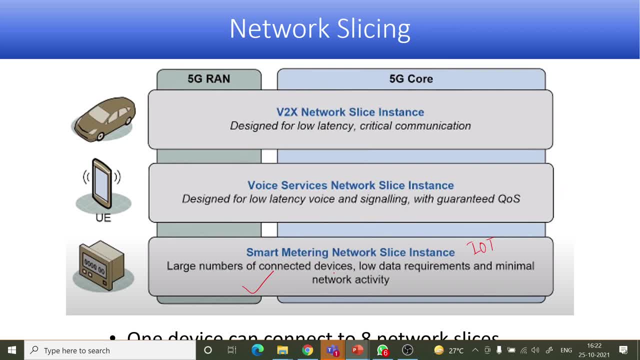 So there can be multiple network slices in a network operator infrastructure dedicated for each of the services and, as per the specification of 5G up to release 16, a user equipment can access up to eight slices at a time. So I mean so normally a user will not be. 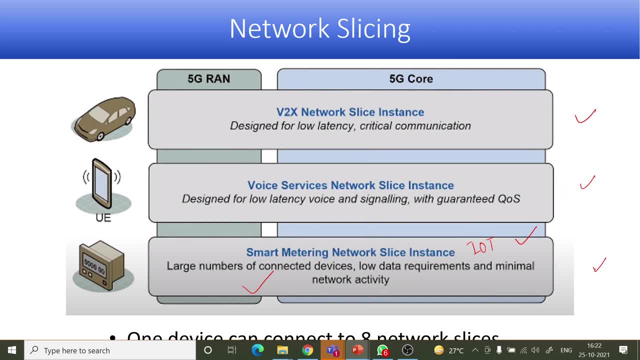 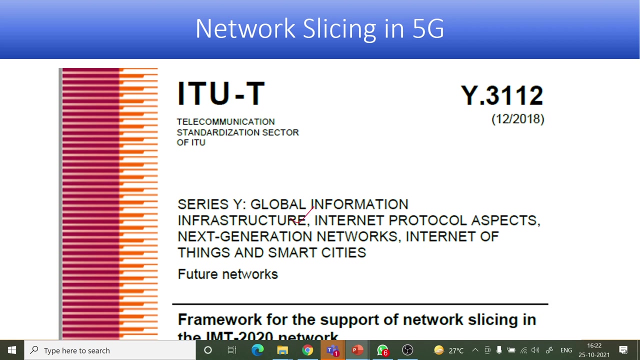 accessing more slices at a time, but up to 8 slices 3GPP has defined that a user can access to simultaneously, whereas number of slices in the network there is no limit. So let us look at the ITU framework. So, as I said, that requirement is normally set by ITU and this document I have shared. 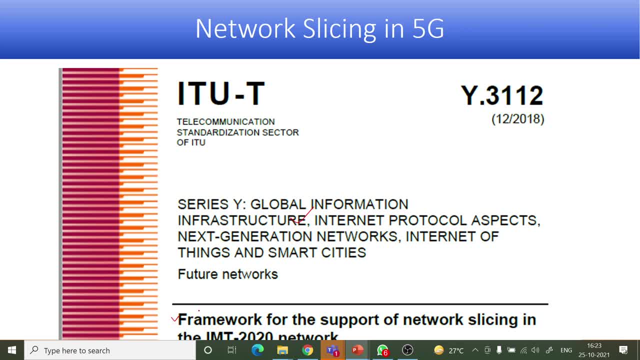 with all of you today in the WhatsApp group. you can read in detail. So this document tells the framework, as I said that earlier- that ITU creates the requirement document and then SDOs make the respective standard. So, based on this ITU framework, everybody is trying to come out with the concept. 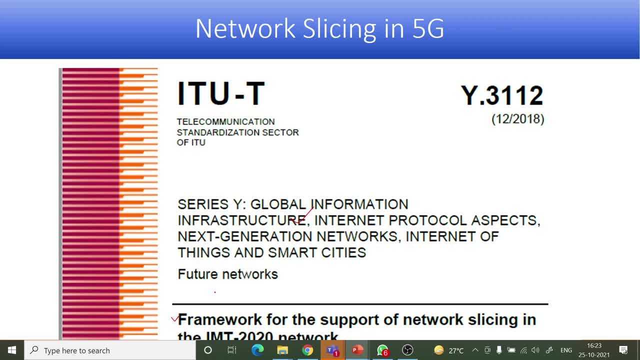 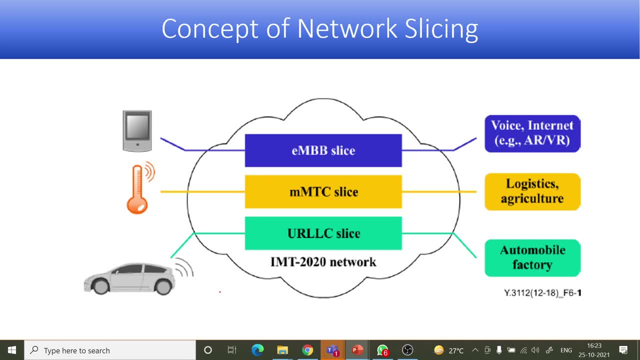 So this was created in 2018, rather released in 2018. they might have taken some years to develop this. So what are those frameworks? So at that point of itself, they had thought of the network, the cloud based network of 5G, which can have multiple slice. they had given example of EMBB slice, MMTC slice and 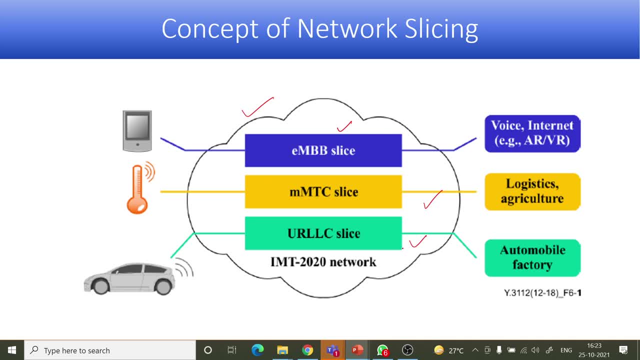 URLLC slice and if you recall that ITU had given these three broad usage scenario- enhanced mobile broadband, massive machine type communication and then URLLC, ultra reliable, low latency communication, So they had also talked about different slice for these applications. So maybe EMBB we use for voice internet, or AR, VR, MMTC for logistics, agriculture, all. 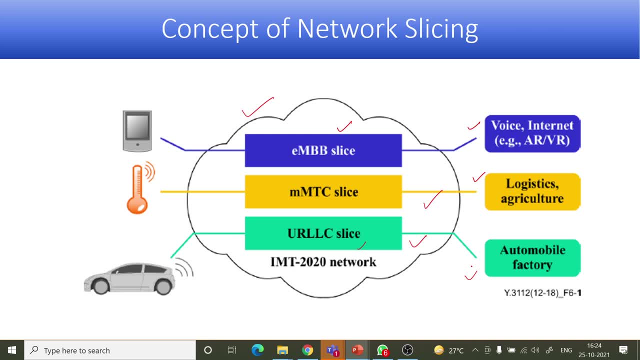 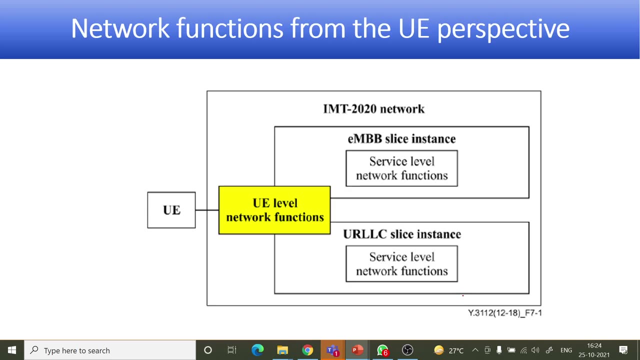 sensor kind of network, URLLC for automobiles, factories, autonomous car and other requirements. So this picture is also taking the same document. so this was the vision for the framework which ITU talked about. Thank you, They had also talked about that. there could be network functions, UV level network function. 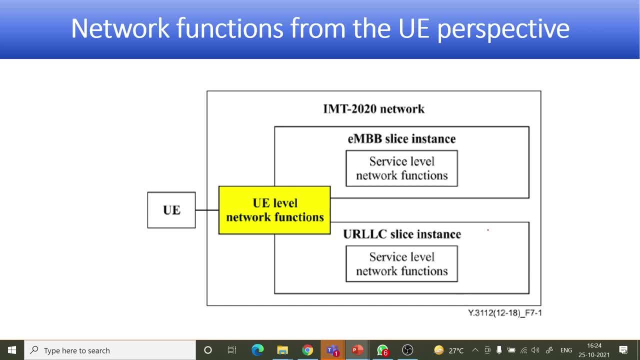 and there could be a network level, service level network functions. So for example, one UV may require to access, say, EMBB and URLLC, right both. So this is kind of a UV level network function. but as far as network is concerned, those slices, 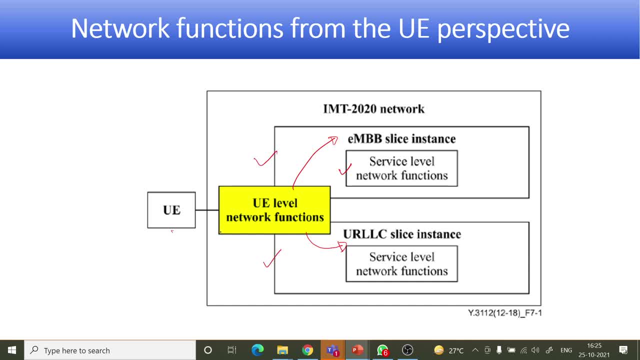 are separated out right, Right. So UV outside can access multiple kind of slices and in 3GPP they have come out is that in the first initial releases up to eight such slices and UV can access two. And then ITU in their framework had given some example, for example in this example: if 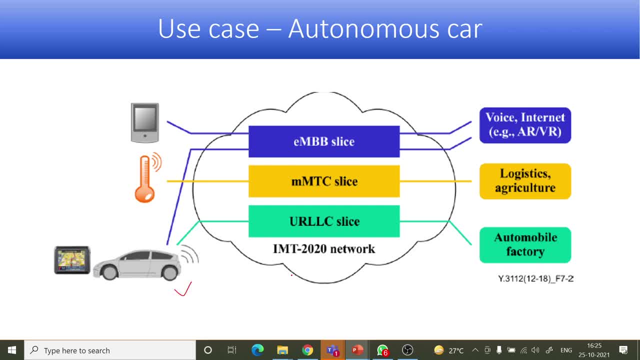 you see this particular application of, say, V2X or automobile factory. it will definitely use URLLC, But it will also require EMBB, So it will be accessing both the slices. So this example says that a UV will be using the multiple slices. 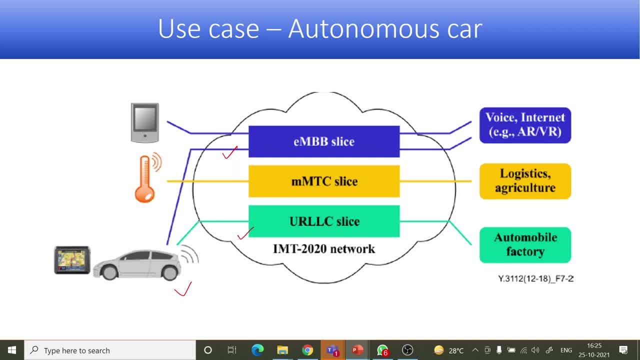 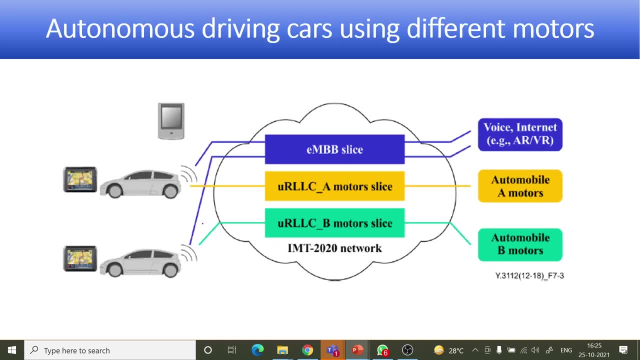 So there are network level- there are two slice- but a service level, it is kind of a one for that particular UV. Again, ITU framework has given document that Okay, So that different kind of manufacturers, for example, it is an autonomous car service which is suppose being given by different automobile company may be. Maruti Suzuki has offered a 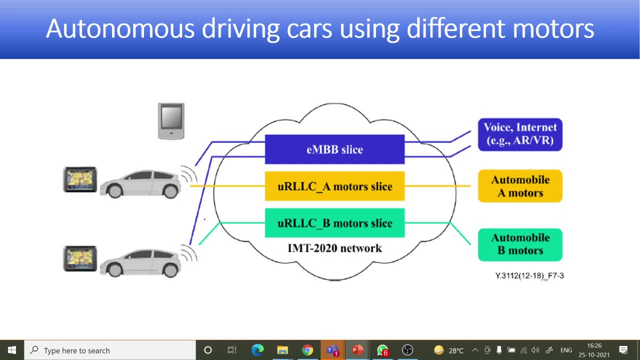 service. may be a Ford has offered a service or may be some other manufacturer. So an operator can create a different slice, different URLLC slice for automobile a motor company or B motor company, But these two motor company will be using the common slice, commonly EMBB slice. 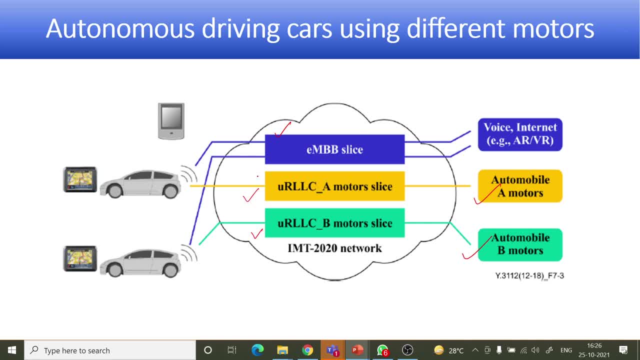 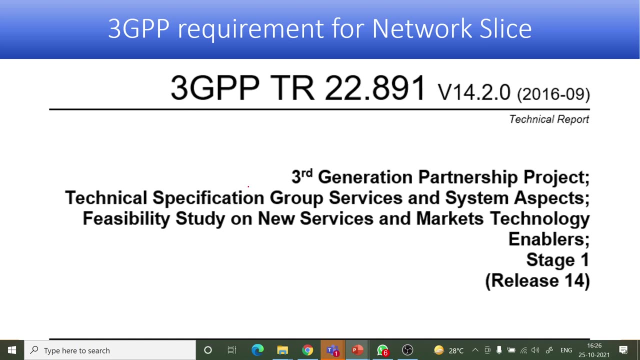 So they have how they have explained in 2018 in their document. you can just understand that all those region had come long back and now I mean just making a standard and making applications are going on. Okay, So those are. those were kind of corrects from the three. 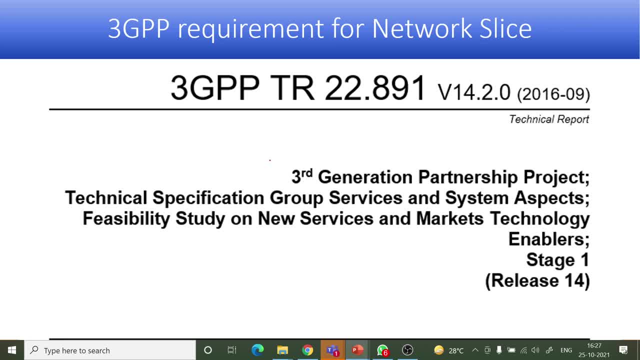 I mean ITU document. now, when 3GPP was working in their release 14 itself- and they are working- they had created a kind of various study documents. So they had done a feasibility study and new services, market technology enablers, stage one, release 14 itself and in this particular document you can download this document from. 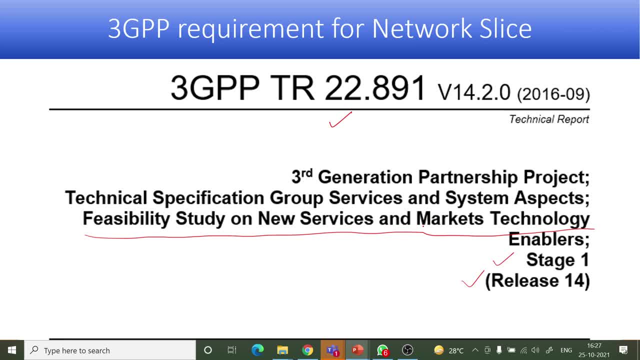 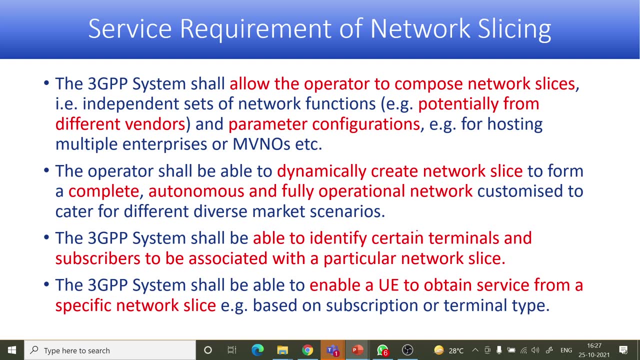 the internet. Okay, So I have talked about certain requirement of network slicing and I will just read out some key portion of those requirement: why I am explaining because how this concept came in and what was the kind of a behind all those visions will come into play. 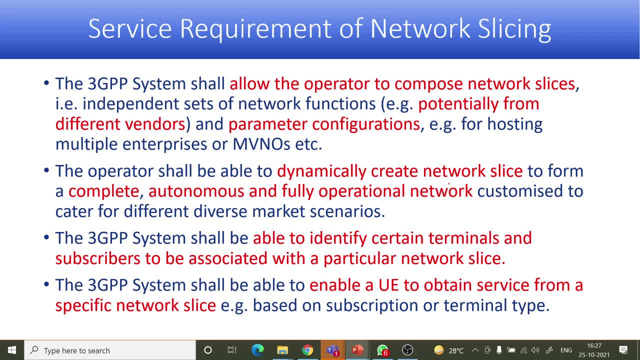 So these are. these are some of the pointers I have taken from that document, So just let me read out some of them. So 3GPP: The system shall allow the operator to compose network slices which will be independent set of network function and that may come from the different vendors. that is the region which 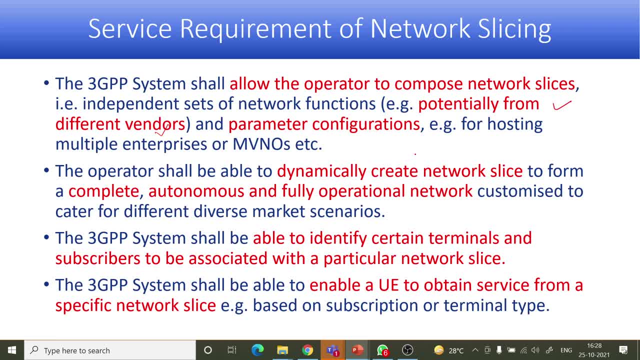 3GPP created and that can be hosted on multiple enterprises right for hosting multiple enterprises, in the sense that those slices can be given to multiple entities, like motor A, motor B I talked about, And then the other requirement they talked about is that dynamically create networks. 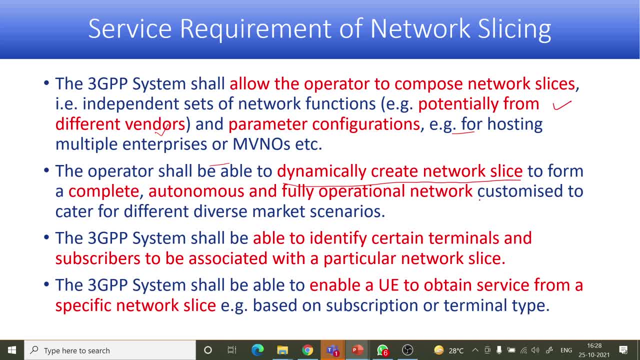 slice. So here comes the importance of the NFB. you have to dynamically create a network slice if you have an infrastructure already- those hypervisors, those containers, environment. So you have to create a slice for a enterprise Immediately, you can configure it. You can configure it. 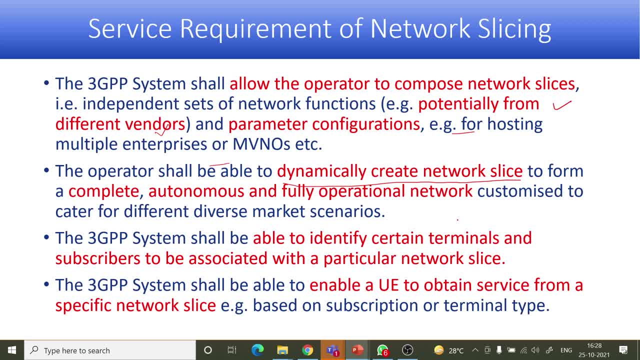 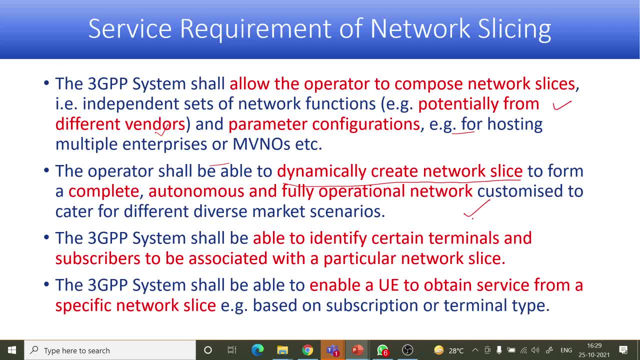 put in the comment, that can be automatically created for a new vertical or new use cases. right, and then 3GPP system shall be able to identify certain terminals and subscriber to be associated with a particular network. slice, So again. So here comes the requirement that I am a user, so which all slice- I am allowed to write. 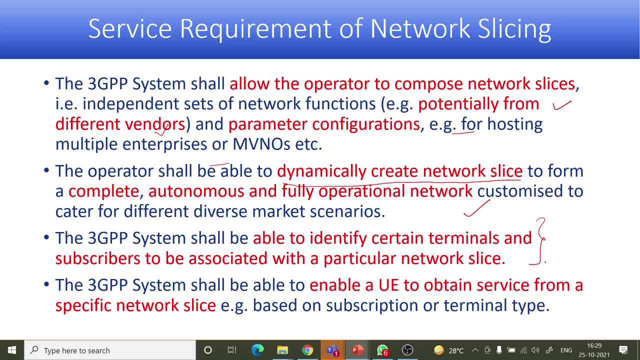 So if I have subscribed to, say, motor A service, I have a car, so then I will be able to access that service. If I am not subscribed, I may not be able to. So I mean system need to identify a terminal and what subscription it has and accordingly 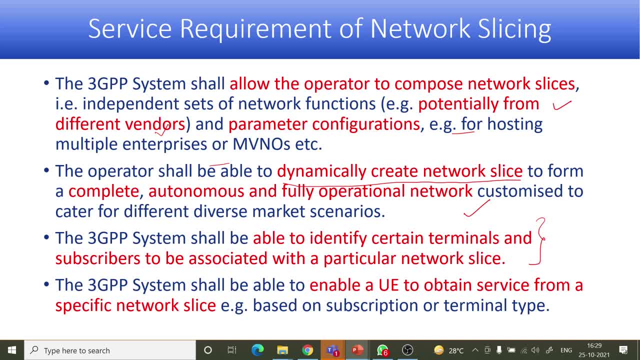 it can allow a service. So that is the requirement which they talked about, And then the 3GPP system shall be able to enable a UE to obtain service from a specific network slice. So same thing from the UE perspective. So these were service requirement of network slicing as envisioned by the 3GPP. 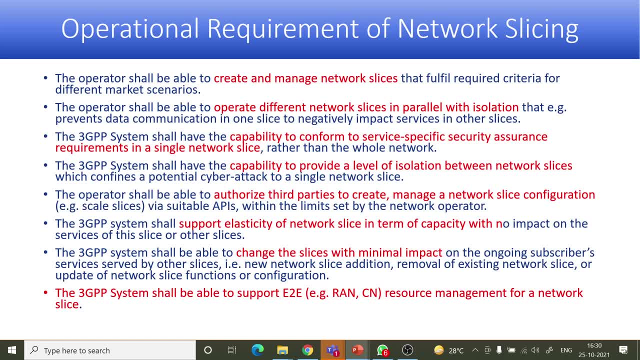 So, based on these visions, they worked out the further specification or they aligned their development to the specification From the operation Operational requirement from the operator perspective. So they talked about operators should be able to create and manage network slices to fulfill the different requirement. 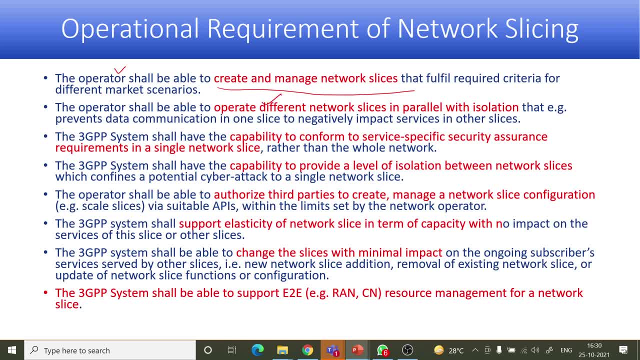 And then these different slices should be able to work in parallel with isolation. When they say isolation that if one slice goes down it should not impact the other slice. So that is the requirement. And then the security assurance part. That means if one slice is compromised, other slice should be completely isolated. 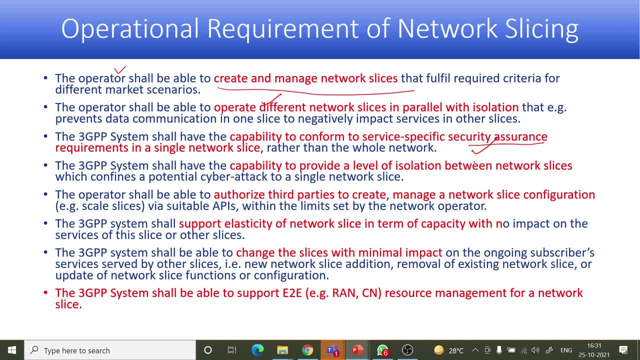 So that you can set down a slice and then continue working on the slice or create a new slice. So it should not affect the whole network. So there is some security aspect also coming in as far as vision and requirement is concerned. So basically, 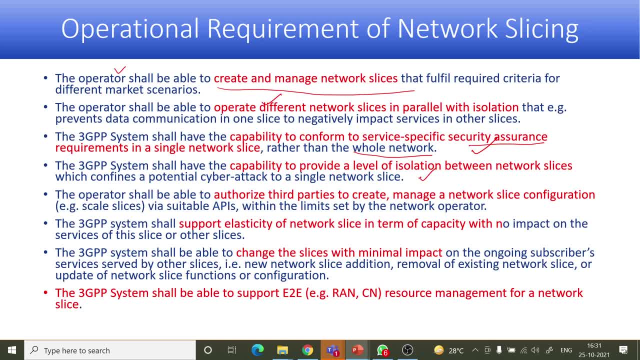 Capability to provide a network. So basically, Capability to provide a network. So this is the level of isolation between network slices, So that whenever there is a cyber attack on a slice, only that particular slice get affected and other slices are not affected. 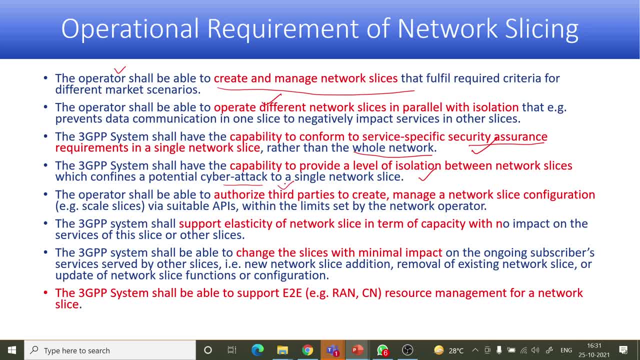 And then operators should be able to authorize third party to create, manage and network slice configuration. For example, if I am giving a slice to MVNO, a virtual mobile operator, then the basic operation should be able to be done by them itself. 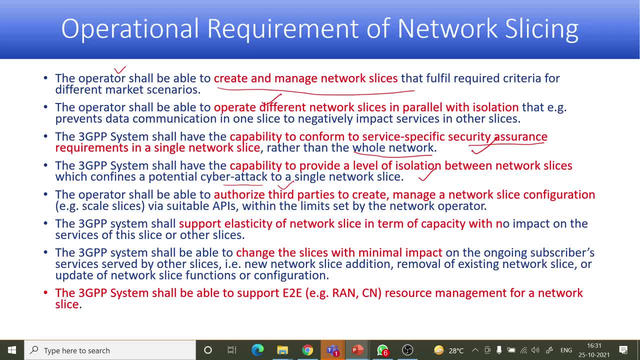 And the overall control will be. the OEM MBNO will get some configurational rights. so maybe with suitable API or whatever way it is possible to be done. And then the next requirement was support elasticity of the network slice in terms of capacity with no impact on the service of this slice. for example, you can increase 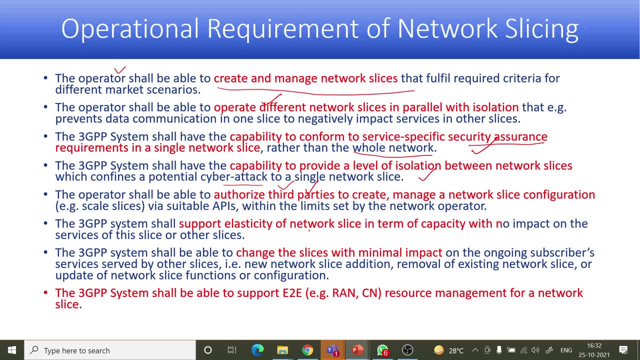 the capacity or decrease the capacity once you have underlying physical infrastructure, NFBI available And you should be able to modify or change the slice with minimal impact. So these were kind of requirement which was talked by 3GPP, requirement document, we can say of that particular study paper. 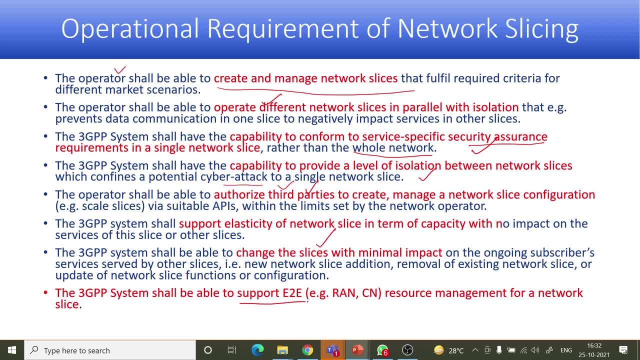 The last point was that I mean it should support end to end Resource management for the slice. it should not be that I am able to manage only the. I am able to manage only the core part and not the rank part. the rank should also be able. 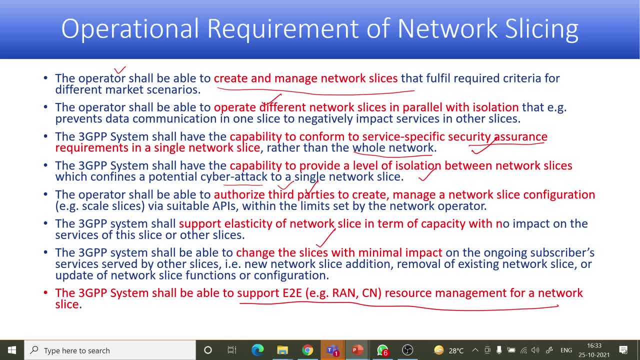 to. we should be able to create slices. Okay, so these were kind of ITU framework and 3GPP vision and 3GPP. after release 14, they came out with the release 15 and 16.. So they aligned all their developments. 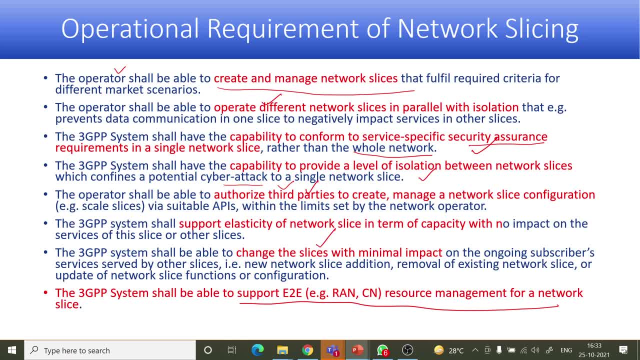 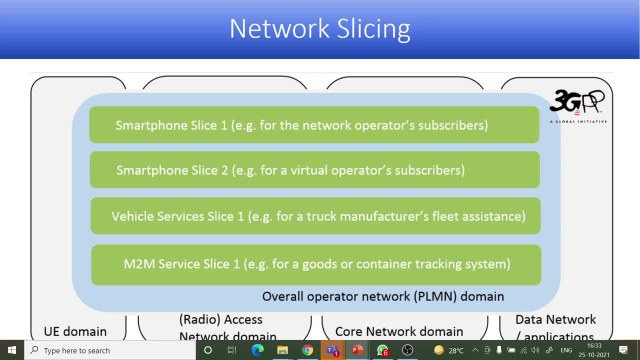 So that it is compatible to the vision which they had talked about. So this particular picture is from 3GPP itself. they have an article on a network slicing, So they have also talked about that. all the domains like user equipment, this is user. 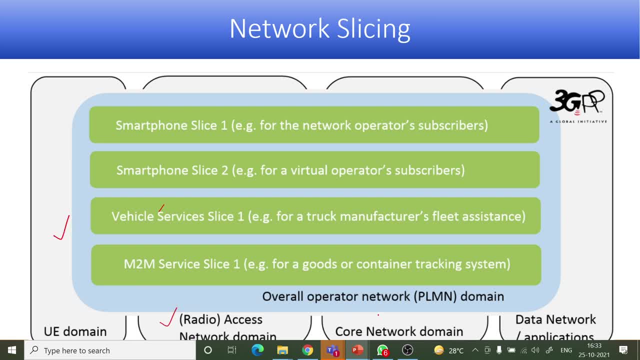 domain. then they are talking about radio network, they are talking about core network function and then finally the data network or applications so combined together. they have talked about creating a slice. so it's not that slice has to be created only in core or only in radio. it is end to end, from user equipment to the services. 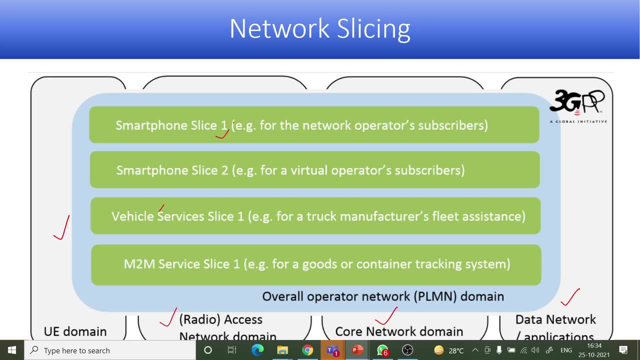 and then they have, they have given example- that smartphone slice. smartphone slice two, i mean one they have talked about one for the operator subscriber, other can be for your mbno virtual operator subscriber. third could be for vehicle slice, the next could be for m2m or 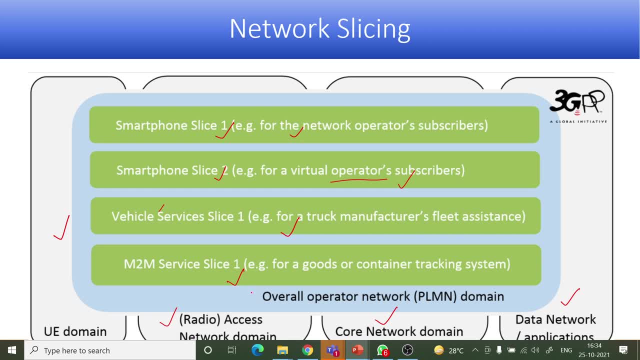 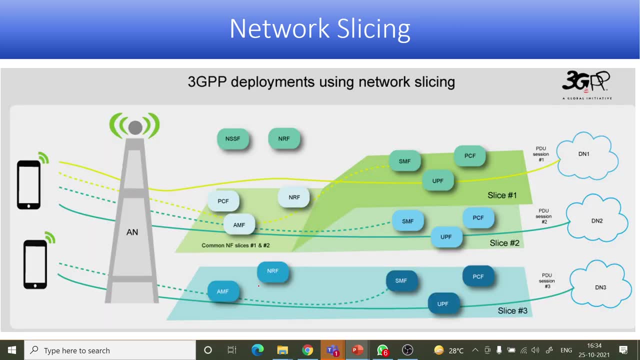 iot slice and so on. so so that is the vision which 3gpp has talked about, and then the network function, as i talked about that. you have to separate out network function for each slice, but there can be some common network function also in this example this is: 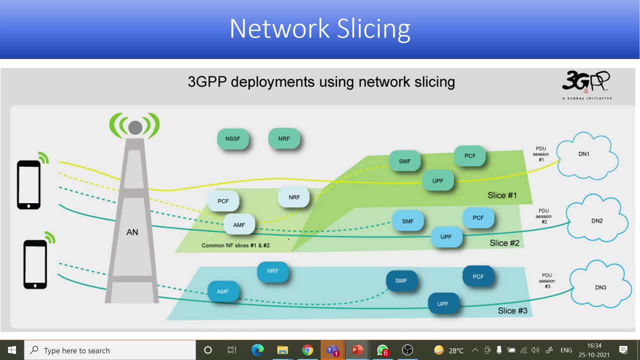 also taken from 3GPP. you just look at that. they have got three slices right. So this is your slice 1,, this is your slice 2 and the slice 3.. Each slice is getting connected to the respective data network, right? So if you look at slice 1, so they have dedicated SMF, dedicated EPF. 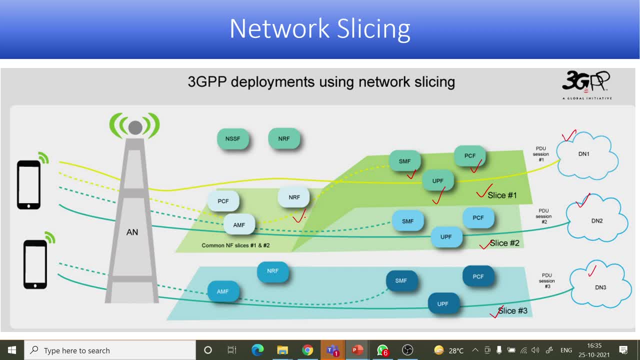 dedicated PCF, dedicated network repository function, dedicated. So here, if you see, I am sorry. So here your NRF, PCF and AMF is not dedicated, but it is common to slice 1 and 2, just see. Just see, it is common to these two. So there are some common network function. 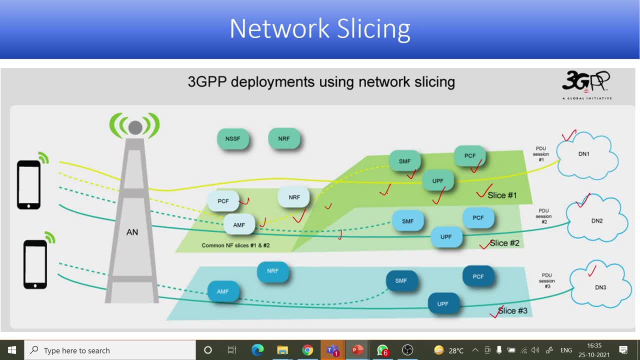 for two slices and there are certain dedicated network function for two slices. In case of a third slice, you see that your AMF, NRF, SMF, PCF, UPF, all are separate as part of the slice itself. In 1 and 2, there are certain common. 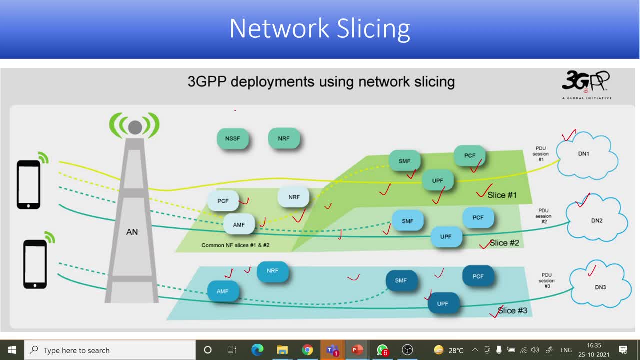 element, and on top of that there are certain common network function, because network slice selection function has to be common, because this only decides which network function to be used for a particular UV, And network repository function, since contain addresses of different network element. So it is a overall network function here. and then you also have 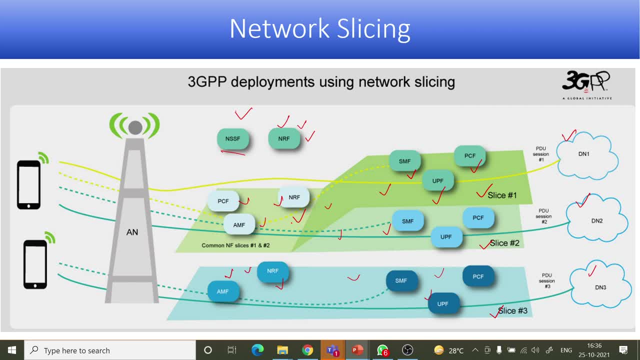 individual network function, right. So individual network function will be there within the slice or common for more than one slice, and there will be overarching network repository function And in the excess network also you have- I mean you need to virtualize or dedicate certain radio resources, may be in terms of frequency. 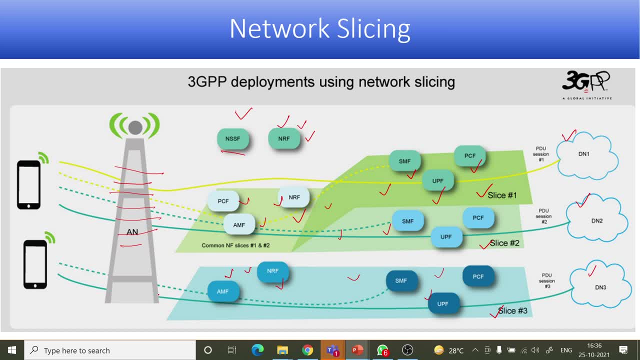 in terms of time and frequency, or in terms of even at protocol layers, how you define. I mean segregate. There are multiple or many ways you can kind of make slice of the radio portion and, of course, on to your backhaul. So the fronthaul, backhaul, midhaul everywhere. 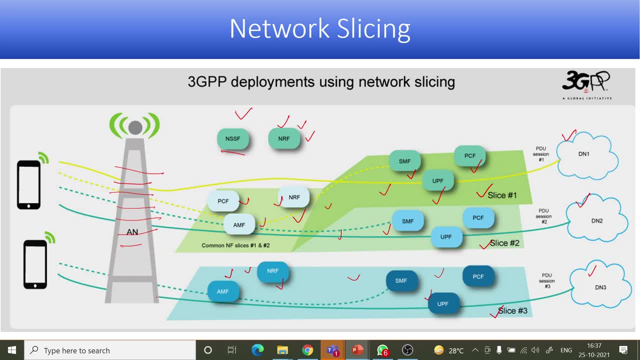 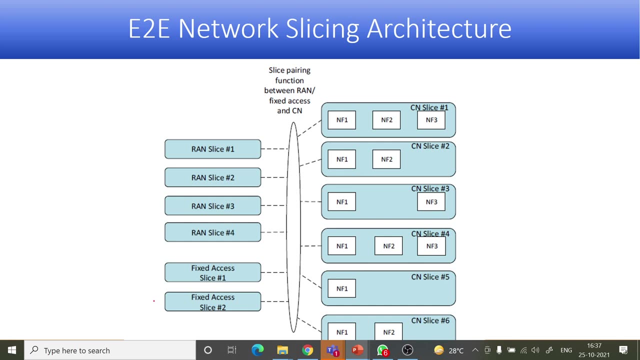 you have to create tunnel for different slicing. So there is a kind of an end to end slicing concept as given by 3GPP. So there are many white paper on network slicing by 5G. America and other GSMA also have given a white paper. you can download that GSMA white paper on network slicing. 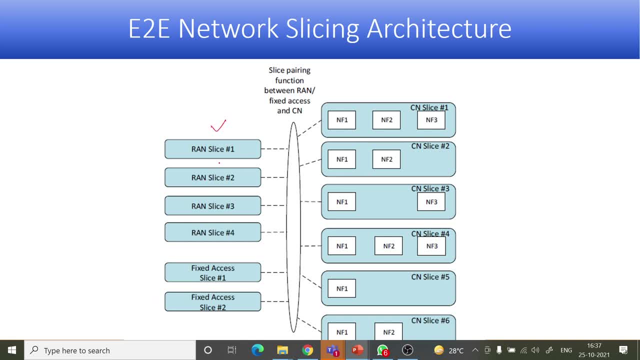 So they have talked about so here also, if you look at that, you have radio network slice, multiple slices of radio network and the fixed network and they go to the core slices onto the core side. you have slice and then you have a mapping. there can be one to one mapping. 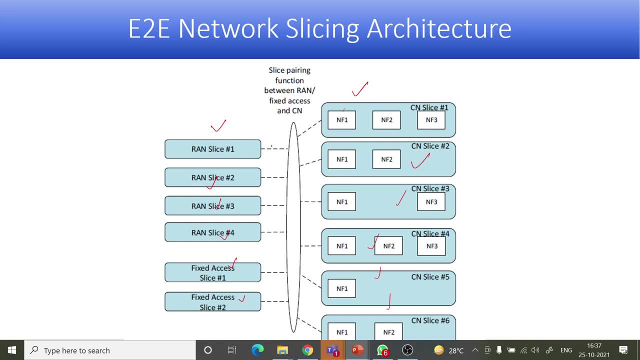 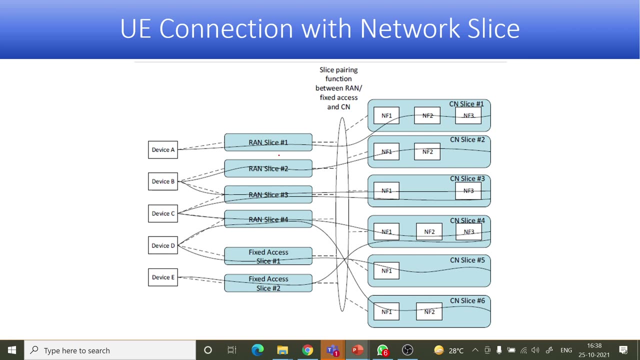 one to many mapping. So there is a mapping that ran slice one may be talking to one CN slice or more than one CN slice and so on. So it is all mapping which is There which can be configured. So here you can see in a detail that a device A is accessing ran slice one and core slice. 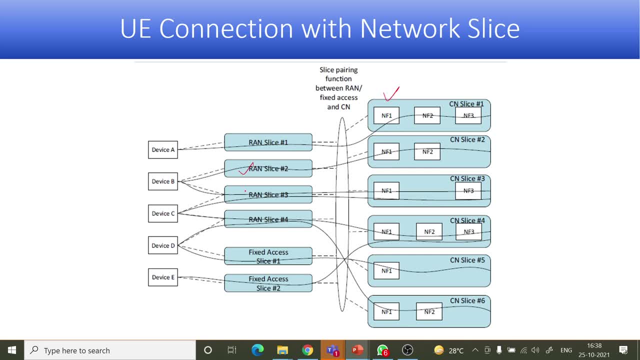 one device. B is talking to two slices of ran and then two slices of CN. So all these things are configurable depending upon subscription of the devices and also different application which can be run. These diagrams are taken from a white paper by 5G. 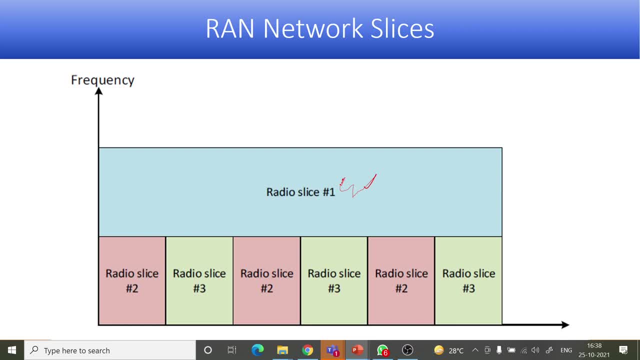 America and there is one paper which has talked about how do you make a slice in the ran part. So one of the example they have given is that radio can be sliced, in the sense that maybe your frequency and time resources, which you talked about, can be dedicated for a particular 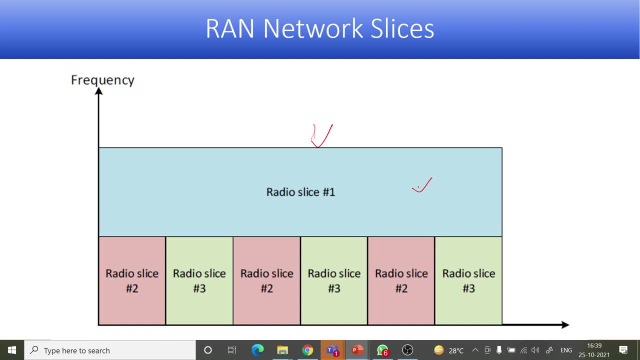 slice, or you can do at the spectrum level. suppose you have two frequencies, one frequency for one slice, other frequency for other slice, So you can do that. So, So, So So there are multiple approaches which will get developed over a period of time, or mix. 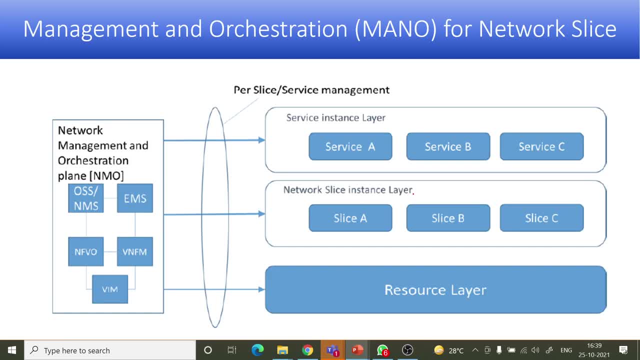 and match will be running. And then the. finally, the MANO part, since network slice requires so many network functions getting deployed in club together. So management of that, you require a management and orchestrations, the MANO. so, so the MANO will create service instance. so what are the service? V2X is a service, PMBBA is service and 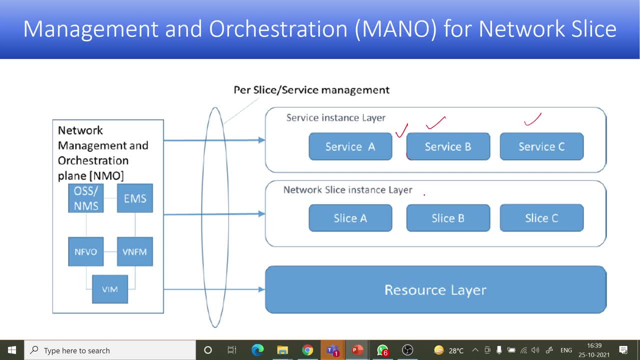 so on, right. so service A, service B, service C, and underlying layer would be that network slice where those resources, network resources, so slice A, slice B, and then you have a resource layer where physical infrastructure we talked about, and there will be a management layer, just like it. see MANO for slices. also those MANO will come into picture. right, because 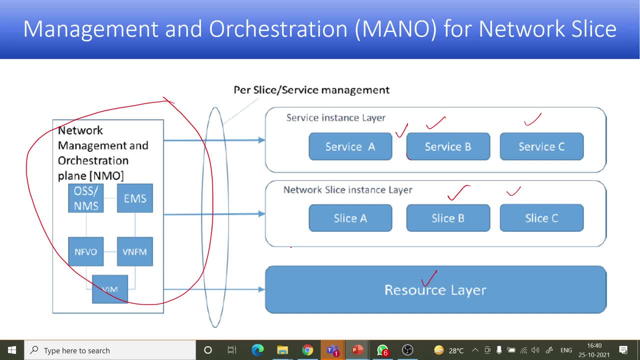 you have to manage the slice very, very dynamically so an MPA becomes a building block or having a network slice. I cannot have a monolithic 5G network and and also the slice. it will be very, very difficult because slices will get created, get modified, get added and deleted for a period of time. 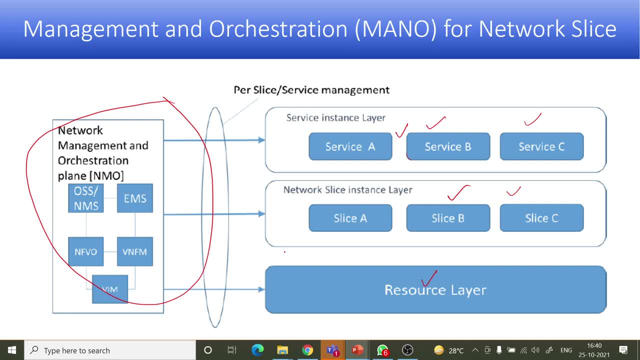 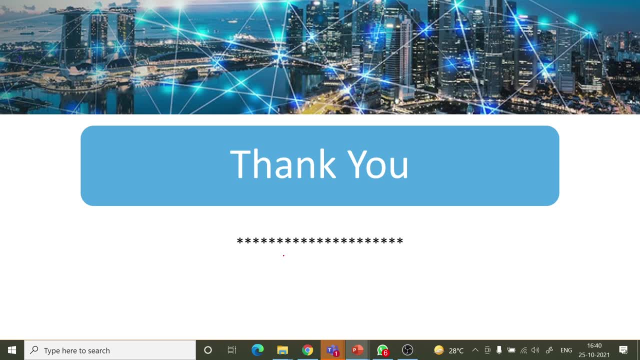 So it's not very, very cost effective to have a monolithic applications. you have to have applications which can be managed. So with this I conclude my session. there is one question I would like to read and answer. can we say one network Slice is equal to one container? 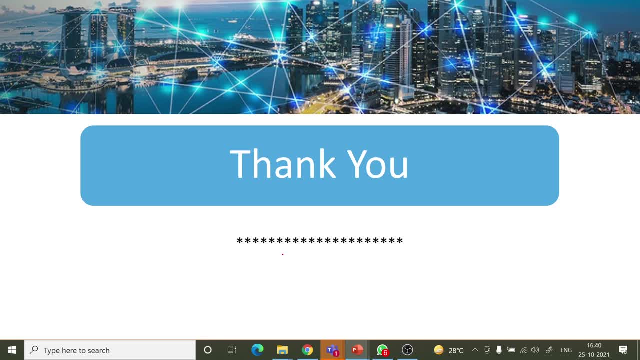 So one network slice may have n number of containers. yes, it's not one container one slice. one container will have one network function, for example. or even one network function can have more than one network. sorry, one container, more than one container, right? So one network function can have multiple VNF.